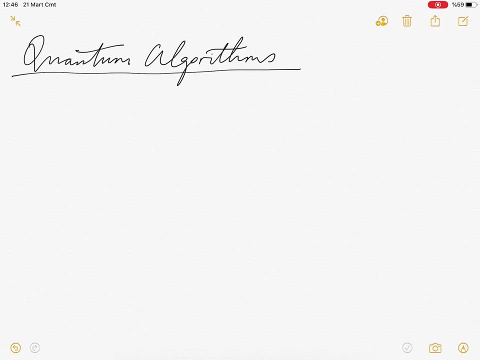 Rather than their summation. So when we take the tensor products, as the size of the system grows, the size of the vector space of the combined system grows exponentially. This is one reason why the quantum algorithms outperform classical algorithms for certain problems, not all, but certain problems. 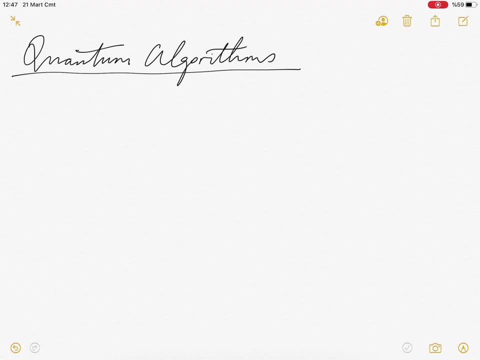 Okay, so today we will start with the most simplest quantum algorithm, Called the Deutz Algorithm. Now, this is perhaps the most simplest quantum algorithm in the literature. The problem is due to David Deutz, Which he introduced in his 1985 paper. 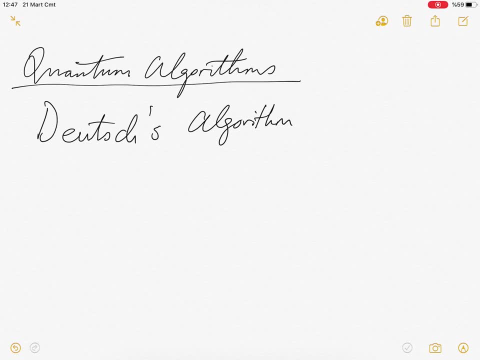 So the problem concerns a function. So a function from 0, 1 to 0, 1 is a function. Okay, so it's a binary function which takes either 0 or 1. And it maps to either 0 or 1.. 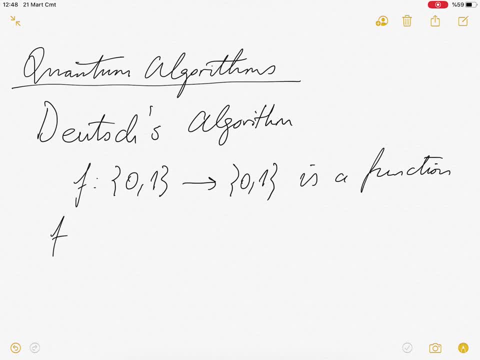 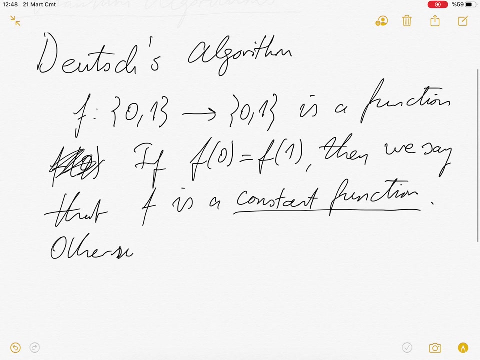 We say that let's define this notion. Okay, so if f of 0 equals f of 1.. Then we say that f is a constant function. Okay, Otherwise. Otherwise, If f of 0. Is not equal to f of 1.. 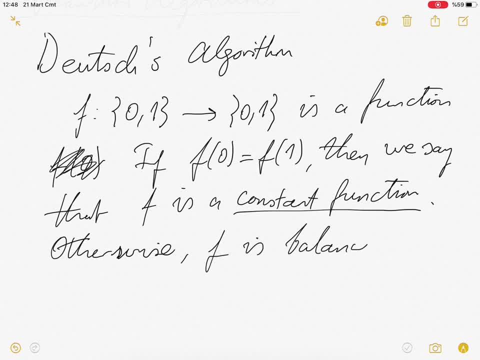 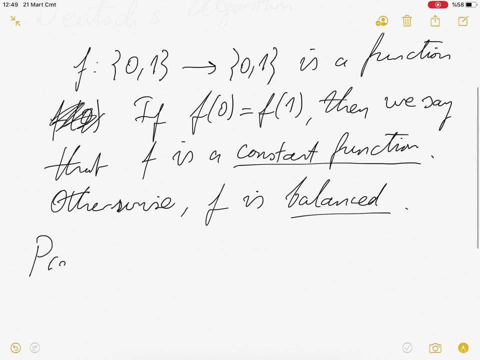 Otherwise, f is balanced. All right. Now the problem is Deutz. problem is Problem. Now given a function f From 0, 1 to 0, 1.. As a black box. Okay, now we're given a function f. 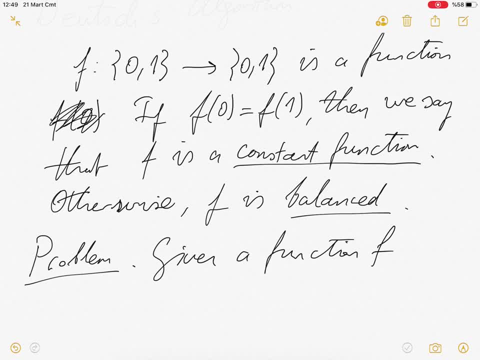 As an oracle, As a black box. We can Evaluate the function f, But we cannot look inside the function. Okay, it's forbidden. So we do not know how the mechanics of the function works. We just, We're just allowed to evaluate. 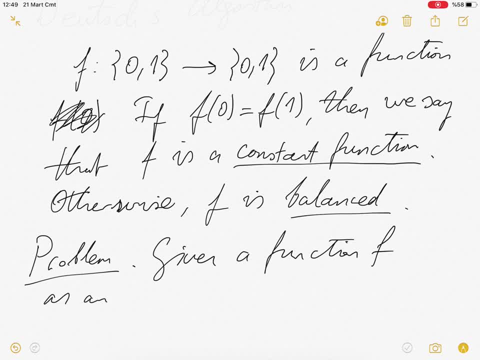 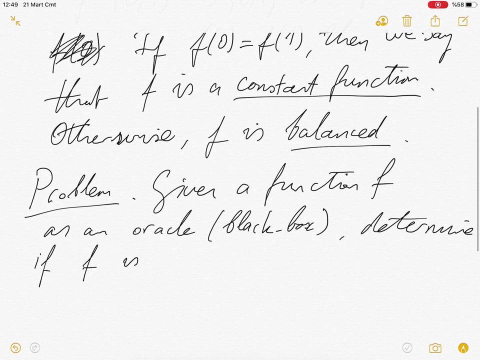 F As an, As an oracle, As a black box. So the problem is to determine if The given function is, If, If f is Constant Or balanced. Okay, All right, So let's think about this problem for a while. 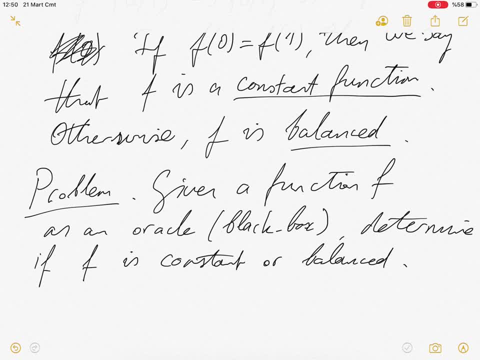 And let's think in terms of classical computers. Now, classical computers Can solve Deutz problem by evaluating f on both inputs, actually on 0 and 1. So we should first evaluate f on 0 and see what the output is. 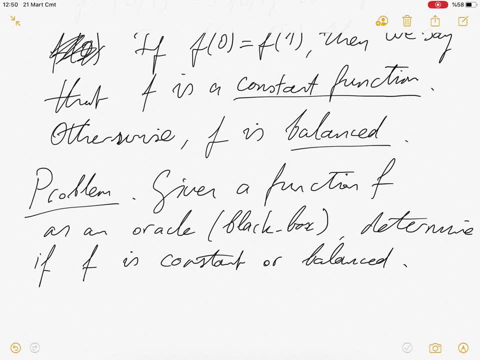 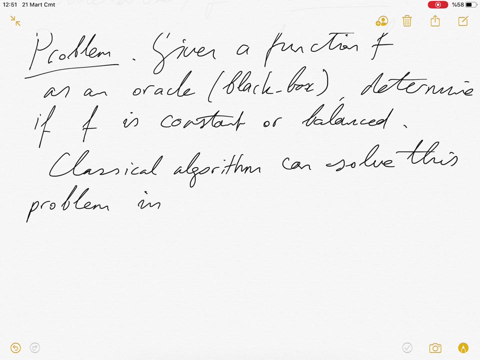 but we should also evaluate f on input 1 and then compare the outputs of the function and tell whether the function is constant or balanced. So we need at least two queries. classical algorithm can solve this problem in well, actually, at most. 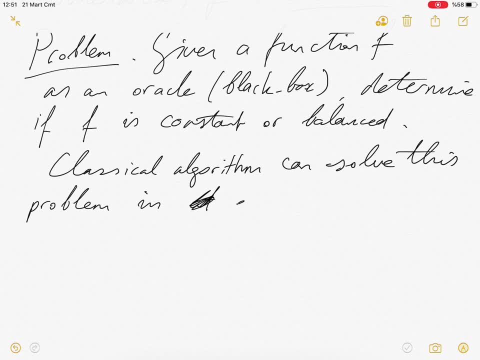 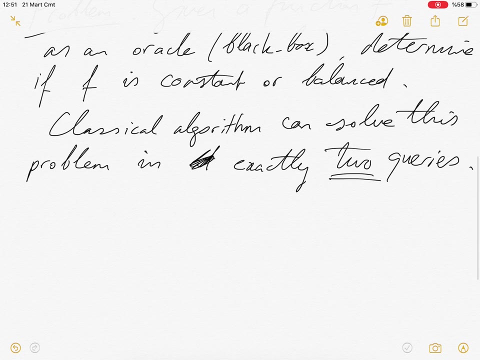 exactly, in exactly two queries. Okay so, but with quantum computing, we will see that we can solve this problem using only one query. Only one query, okay. So before going into the details, let's describe how we can define a function f in terms of matrices. 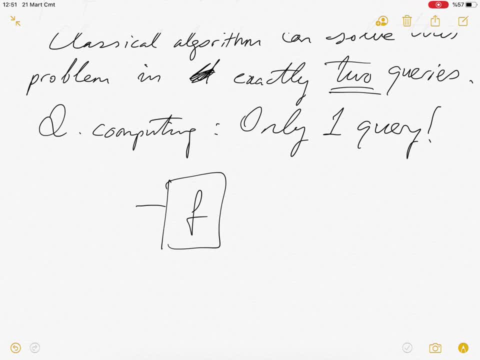 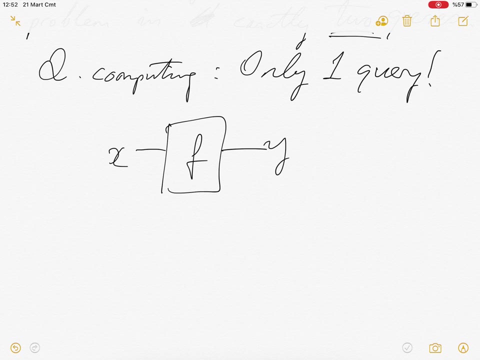 Now classically defined. a function can be thought of as a black box. okay, having an input and an output: x, y. this is a classical representation of a function, and a one-bit input and a one-bit output function can be represented by a two-by-two matrix- okay, 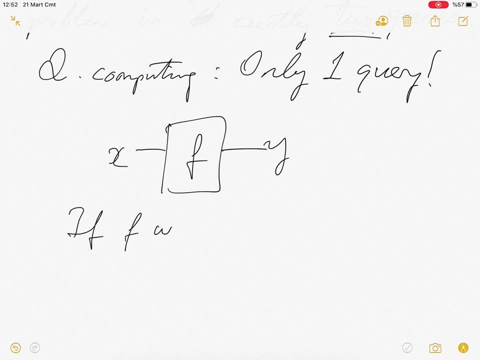 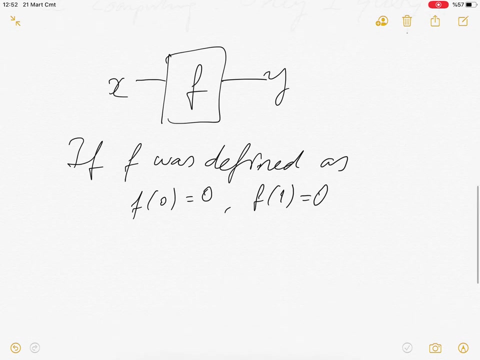 For instance of a function, if f was defined as something like you know, if f0 was 0 and f1 was 0. So if f was a constant function, then I could represent f by the matrix 1, 0, 1, 0, right. 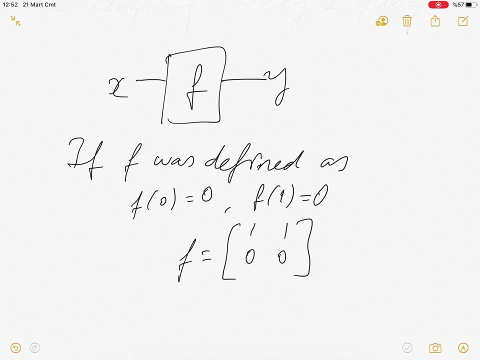 So it maps ket 0 to ket 0, and it maps ket 1 to ket 0. It's a constant function And this. you can see that it's a constant function. So this would be the matrix representation of the function f. 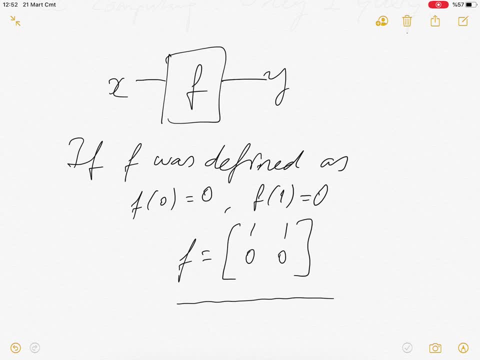 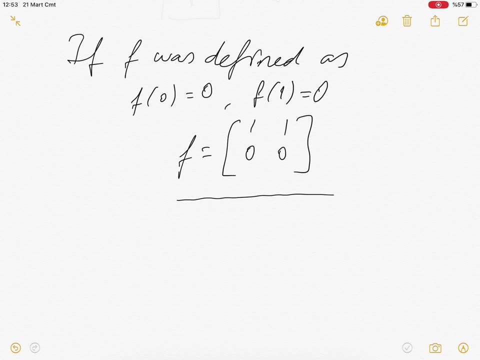 Okay, Now we call that quantum systems. In quantum systems, we require all our functions to be unitary, hence reversible. So we need to make this function reversible. And let's suppose that f is given as a block box, but in terms of 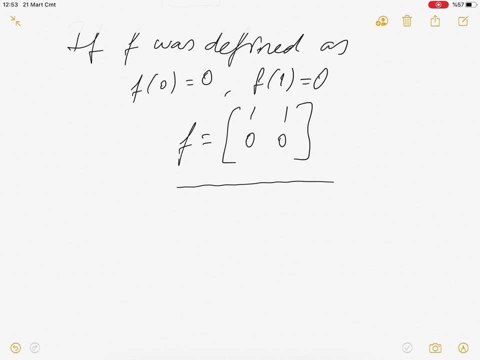 in terms of, in terms of its quantum counterparts. okay, So let's call the quantum counterpart of f uf. okay, So this is the quantum counterpart of the function f. All right, Now uf will be given as an oracle. 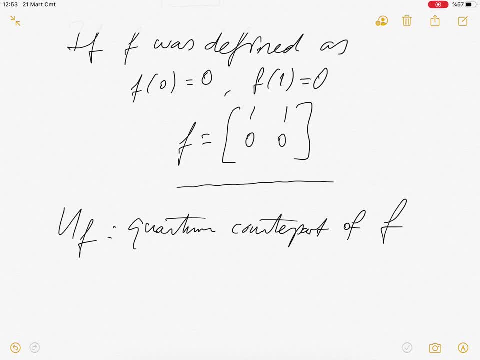 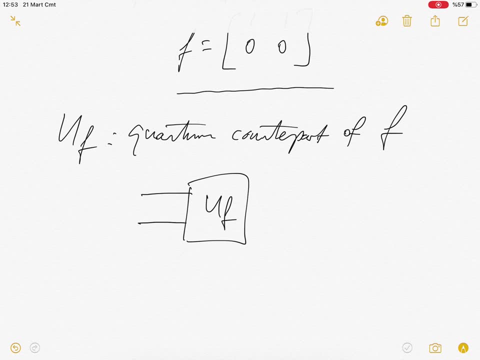 and it will have two inputs and two outputs. It will give, it will be given as an oracle and it will have two inputs and two outputs. So it will be given in the form of a block box like this. It will have two inputs. 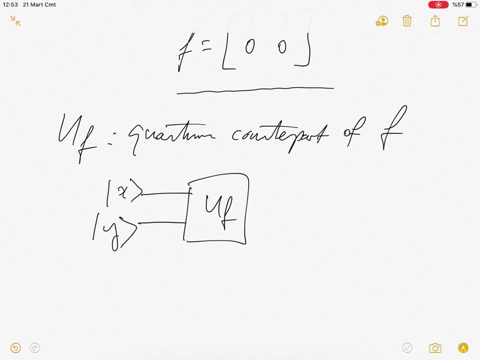 ket x. This is ket y. Well, the first output will be will be the qubit that we want to evaluate. Okay, So x will be the qubit that we want to evaluate and y here controls the input And then in the output. 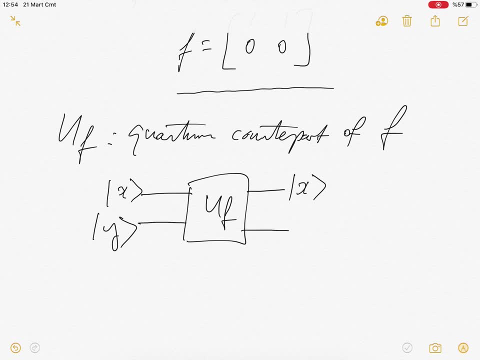 we have x, and the second qubit of the output will be y. Okay, So this is. we have exactly what we want to evaluate. In summary, we're going to look at x, v, y, y, x or f of x. 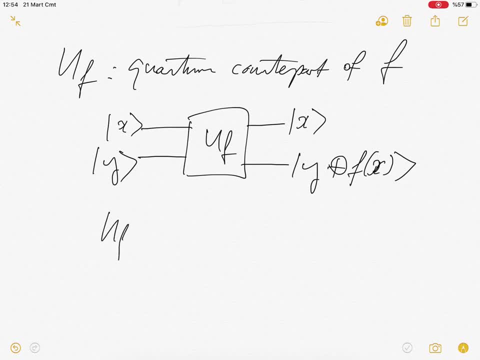 So, in summary, uf takes the state x, y, a two qubit state and it maps to x, y, x or f of x. Okay, So this is this: is y, x, y, x or f of x? 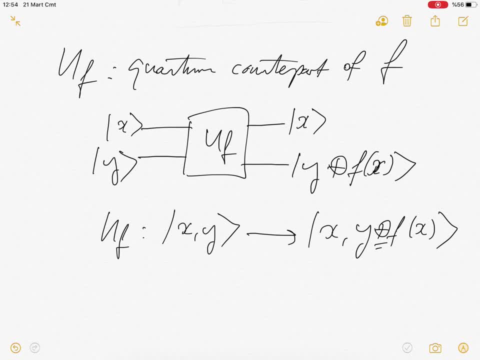 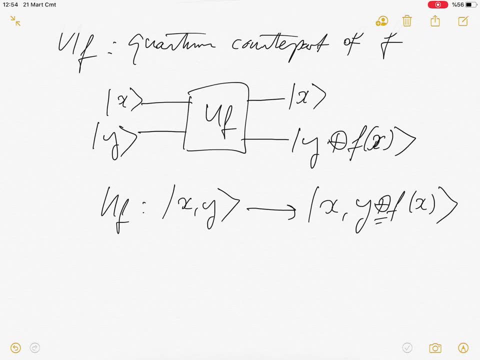 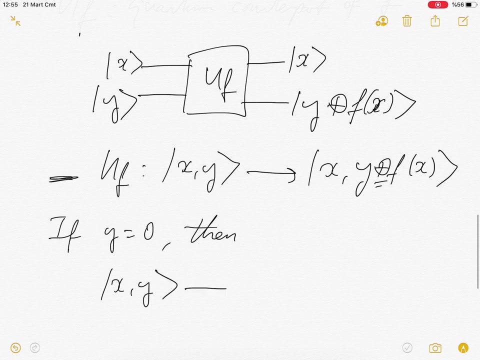 So this operator here is simply binary XOR. okay, All right. so, furthermore, if Y equals 0,, then this expression simplifies to: if Y equals 0,, then the above expression simplifies to: so XY will be mapped to X 0, XOR F of X. okay, 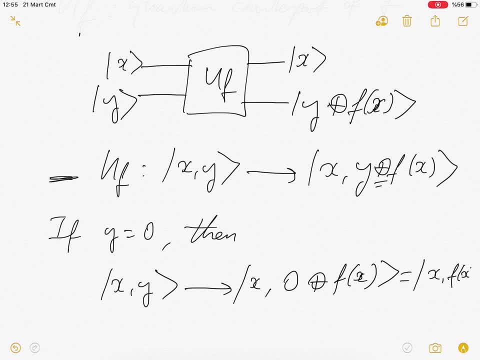 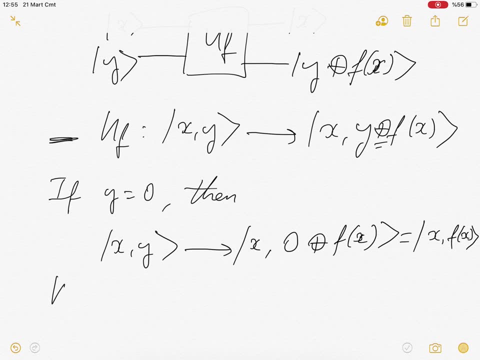 But this is simply X, F of X. Now you can easily notice that UF is reversible. Okay, that is, if we give, if X, Y, XOR F of X is an input to UF, then the output will be XY. okay. 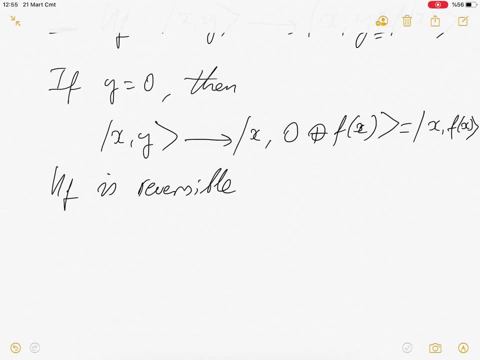 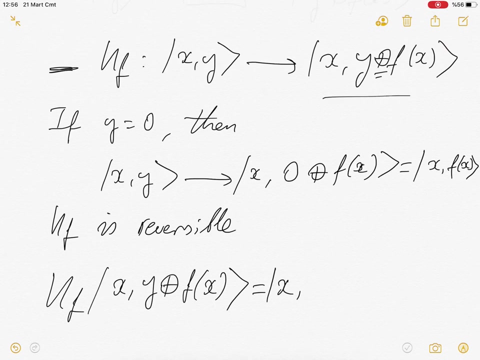 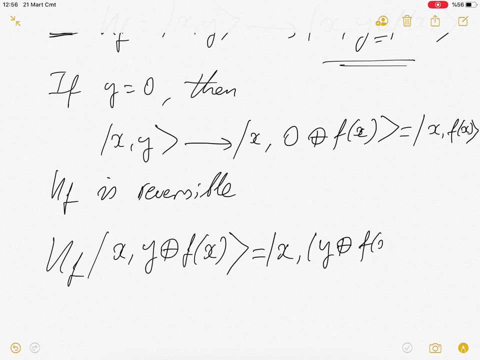 So let's see that in fact. So if the input to UF is XY, XOR F of X, okay, so this will output X, I'm taking. I'm applying this function here, so it will be Y, XOR F of X, XOR F of X, okay. 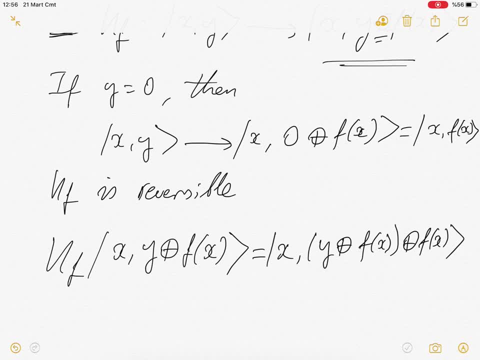 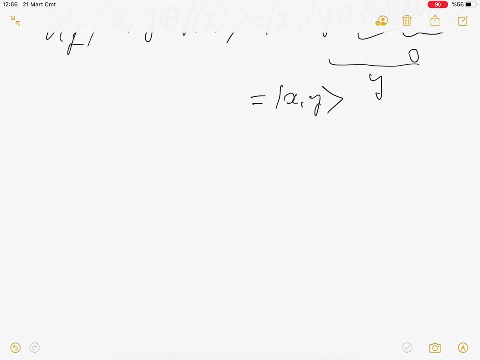 Now we know that F of X XOR F of X is simply 0.. Y XOR 0 is simply Y, so this will be equal to XY. Okay, so let's consider the function. let's consider the function F, defined as as follows: 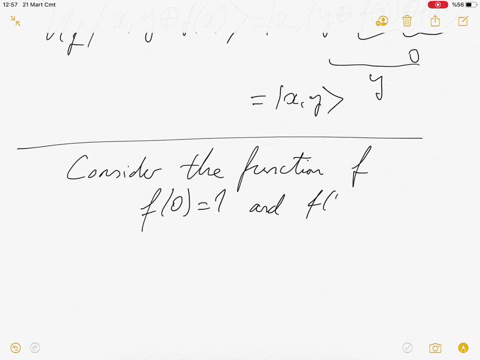 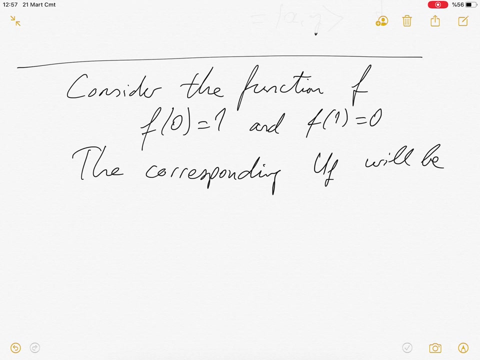 F of 0 is 1, and F of 1, F of 1 is 0,. okay, so it's simply the the NOT function. Now the corresponding UF will be: will be defined by the following matrix: okay. 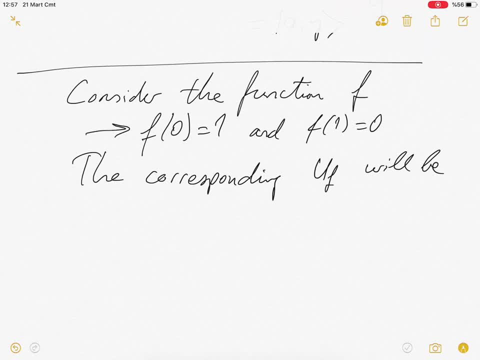 So if we take this function, then the corresponding UF will be equal to the matrix. so it will map. it will map the state 0, 0 to state 0, 1, right, So the first column of the matrix will be 0, 1, 0, 0.. 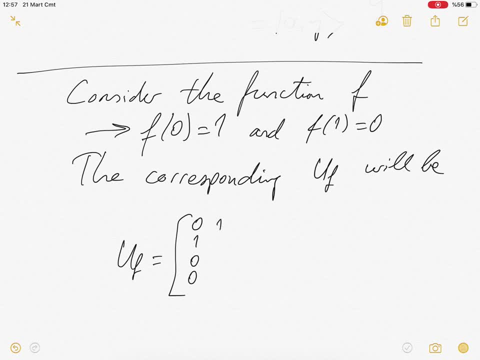 It will map 0, 1 to 0, 0, and the third column will be 0, 0, 1, 0,. the fourth column will be 0, 0, 0, 1.. So when you give 1, 1,, 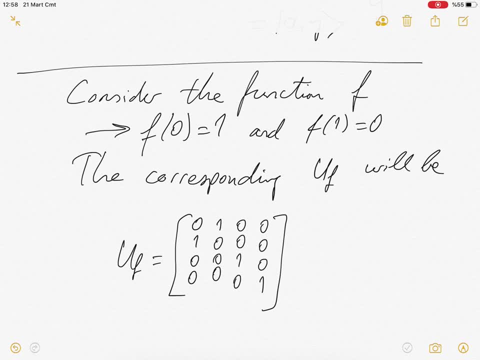 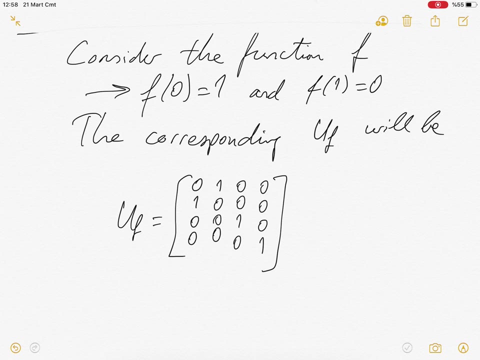 as an input, the output will be: oh, I'm sorry. yes, if we give 1, 1 as an input, the output will be the same. Okay, so now the problem is to determine whether UF is a constant function or a balanced function. 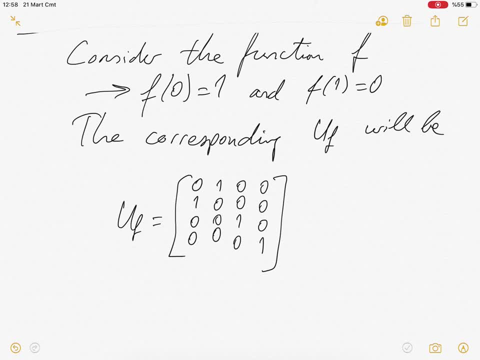 Okay, so we're given the function F, given in terms of a given in terms of its quantum counterpart, UF, given in terms of a given in terms of its quantum counterpart, UF, and the problem is to determine whether UF is a constant or a balanced function. okay, 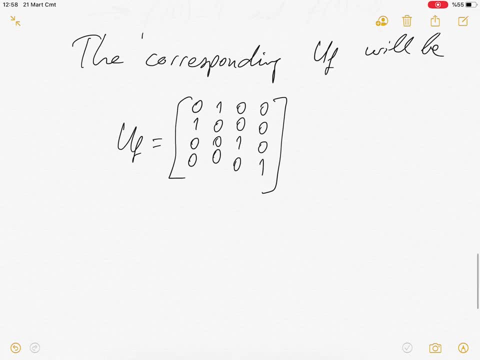 Okay, now we will. we will use the circuit method to describe our quantum algorithms. There are other methods that we will discuss later on, but for simplicity, we will start with the circuit, the circuit model, and it's similar to what we did when we 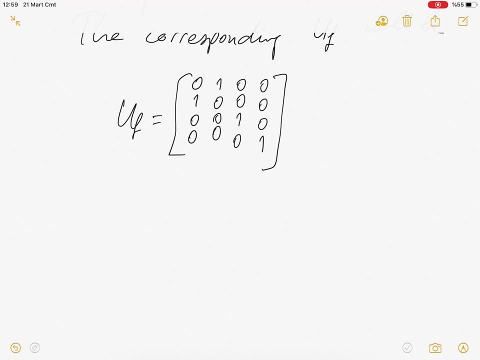 when we generated the EPR pairs. Okay, is now we? now we, we. we draw some wires and we used Hadamard transform the CNOT gate, And we're going to use a similar approach here. Now, our first attempt. 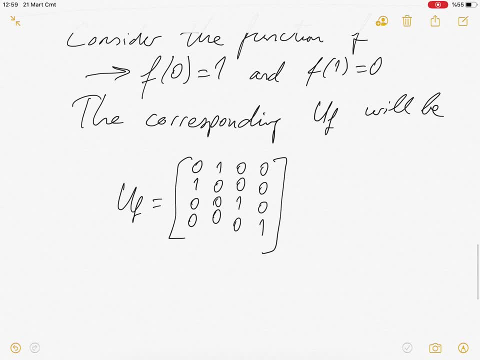 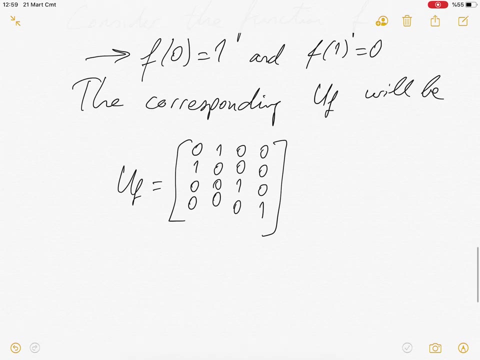 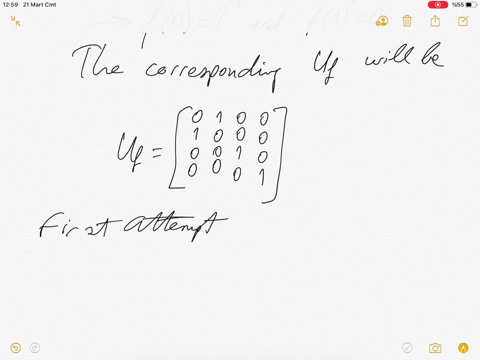 rather than evaluating F on different inputs. so, rather than evaluating F twice, let's actually put the input states into superposition. Okay, This would be the most natural approach in a quantum algorithm. So, as our first attempt, Okay, first attempt. 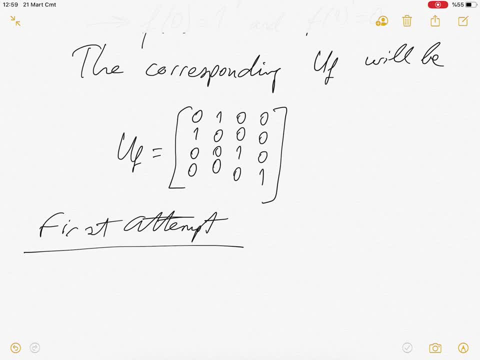 Now I'm going to give you the wrong solution, by the way. okay, I'm going to give two wrong solutions and one correct solution in the end. All right, so we try to put the inputs into a superposition, All right? so, instead of 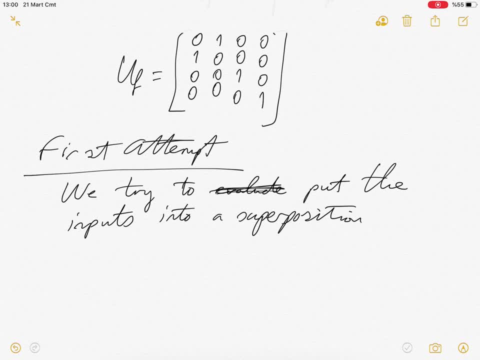 having the top input to be either in state 0 or 1, we put the top input state in this plus-phase superposition state. okay, So we put the top qubit of Uf in state ket 0 plus ket 1. 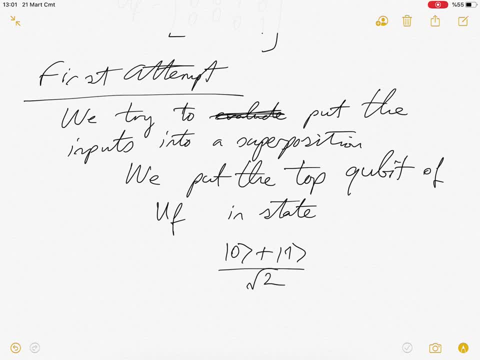 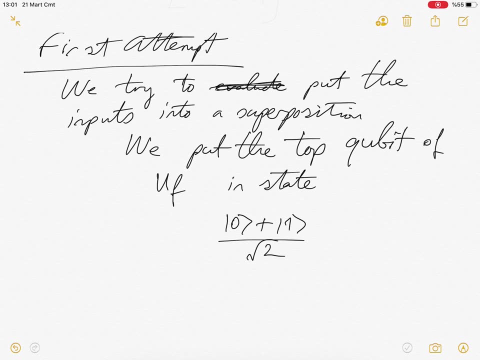 divided by ket 1.. Okay, so we start with the input ket 0 and we apply the Hadamard transform to ket 0 and then obtain this superposition state right. So because Hadamard 0 is equal to 1 over square root 2, 0, 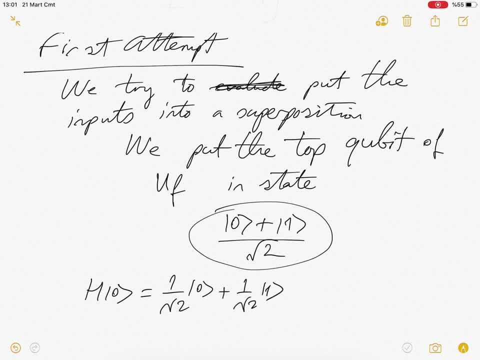 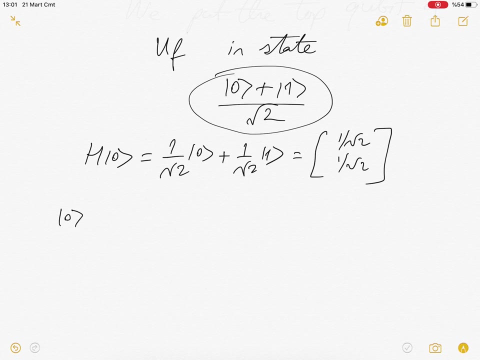 plus 1 over square root, 2: 1, okay, Which is equal to this vector. All right, so let's draw the circuit diagram. We start with: the top input will be set to 0, and then we have a Hadamard transform here. okay. 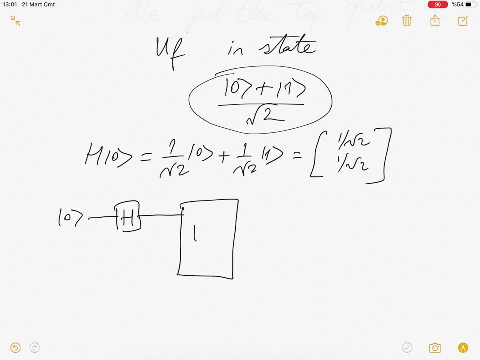 This will be the first input of Uf and we basically set the second input to ket 0,, okay, And then we have two qubit outputs And then, in fact, let's measure the first qubit. here I'm going to use this notation: 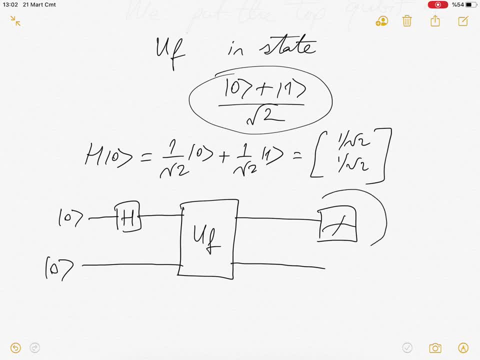 to denote measuring. okay, All right, so let's divide this into stages. Suppose that this stage is denoted by phi 1.. Let's call it phi 0, okay, It's phi 0 in the notes. Let's call this stage phi 1.. 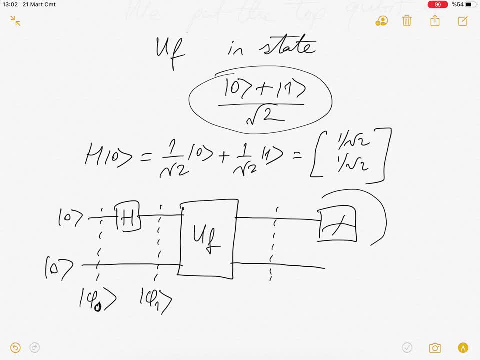 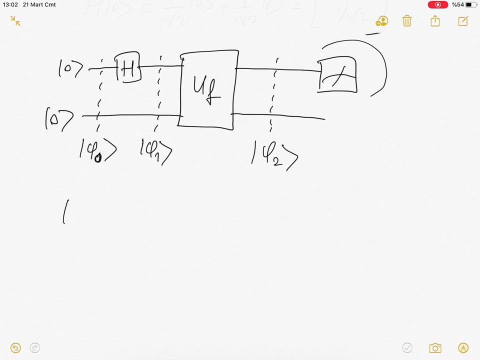 And let's call the final stage the output of Uf two, qubit output. let's call this phi 2.. Now let's look at each state and how they're defined. Okay, so it's easy to see that phi 0 is simply 0, 0, okay. 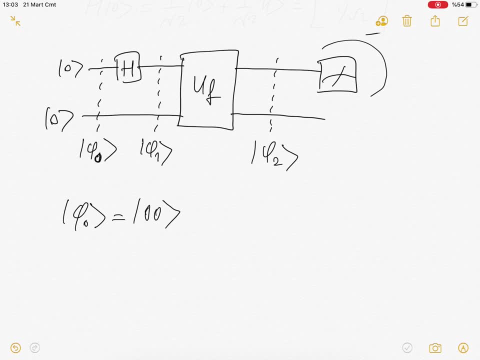 The first qubit is on state 0 and the second qubit it's in the same state. So this is straightforward. Phi 1 is when the first qubit is put into superposition, So the first qubit is in state plus 0,. 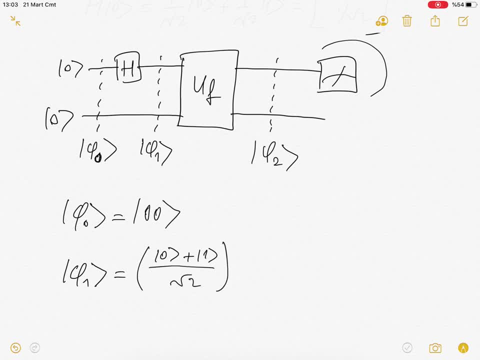 0 plus ket 1, divided by square root 2, tensor ket 0,. okay, Now, this is the first qubit in a superposition right And this is the state of the second qubit, which is unchanged. If we distribute it, we get 0, 0 plus 1, 0. 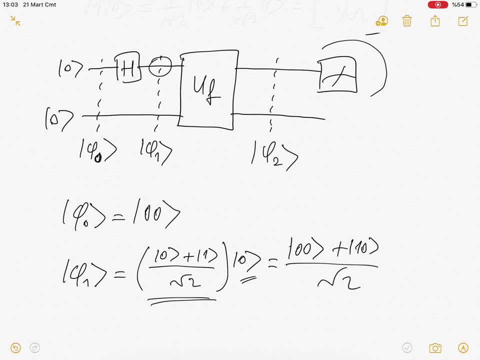 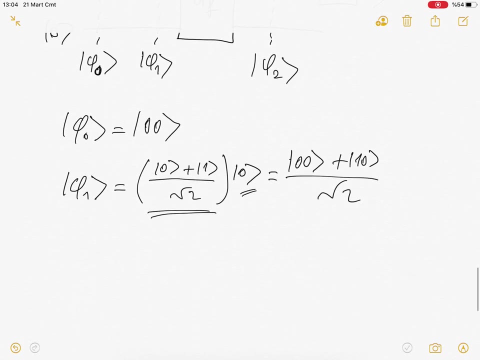 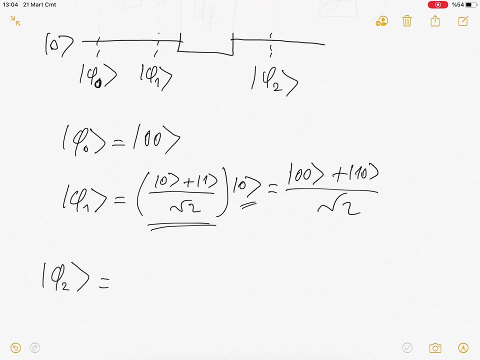 divided by square root 2.. All right, now it's time to apply the function Uf on phi 1.. Now Uf is a linear function, So okay, so phi 2 will be actually. so we have Uf 0, 0 plus Uf 1, 0, okay. 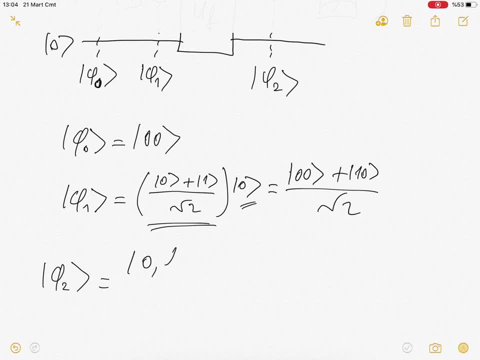 But then we have as an output we have 0, f 0,. okay, If we apply Uf to the first component and in the second component we have 1, f of 1 divided by, we have the 1 over square root, 2 amplitude. 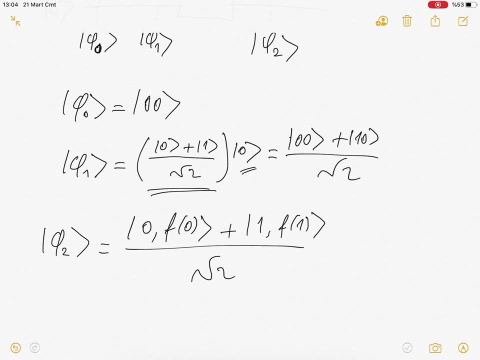 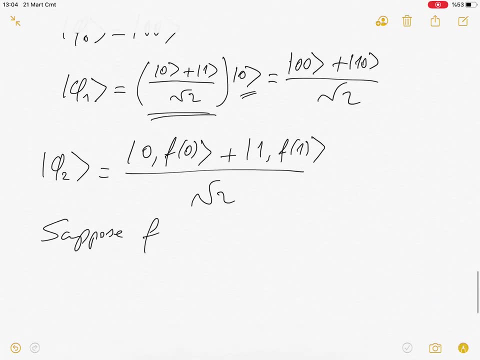 Now, let's suppose that our function was defined as earlier. Suppose that f of 0 is 1, and f of 1 is 0. Let's think about the worst. Let's think about the worst case scenario, okay, Because we want to have a general solution. 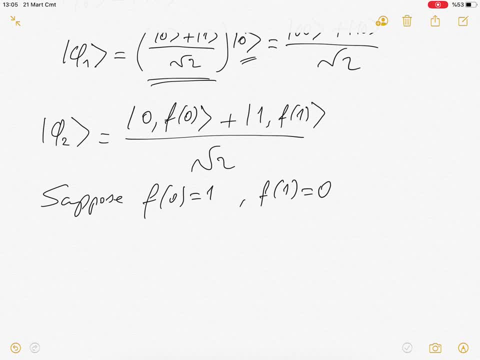 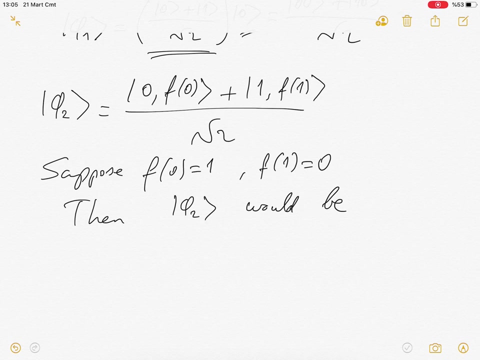 Okay, if f was defined in that way, then the state phi 2, phi 2 would be, so I'm rewriting phi 2.. So it will be basically 0, 1 plus 1, 0 divided by square root 2.. 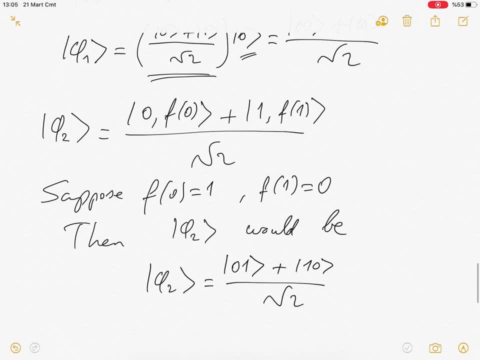 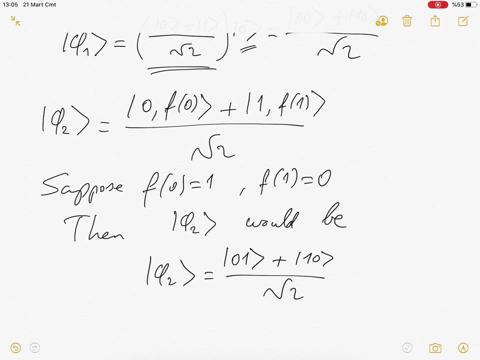 Okay now what do we get out of this? If we measure phi 2, the first qubit will be in state either will be in state 0 or 1, each with probability 1 over 2, actually right. 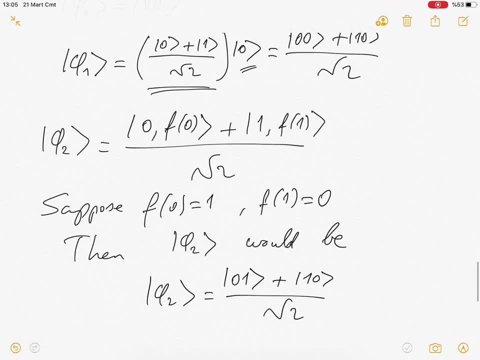 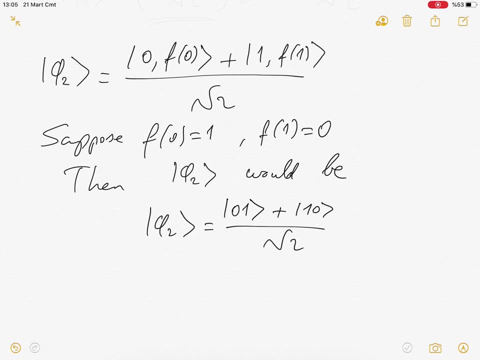 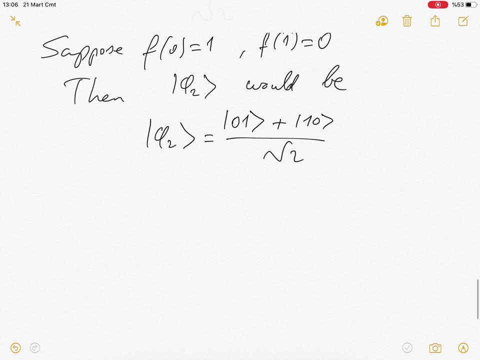 So we get nothing. We have no information about whether the function is constant or at balance, And similarly for the second qubit. there's an equal chance of the second qubit being in state 0 or 1.. So now we should devise a better algorithm. 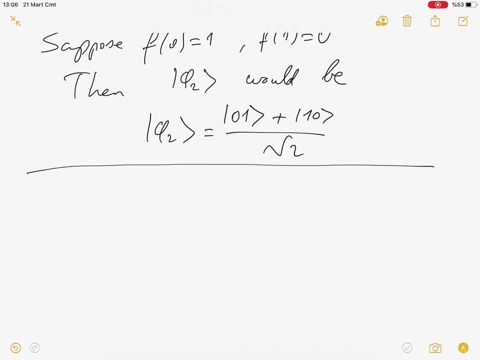 So the first attempt fails? okay, We have no information about the function f. As our second attempt, we have no information about the function f. Okay, rather than leaving the second qubit in state 0, let's put both qubits in a superposition state. 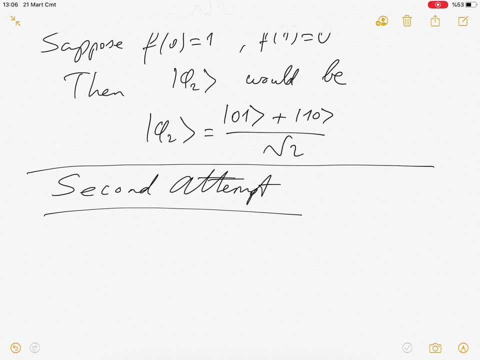 except that, oh, actually, we leave the first qubit arbitrary, But we put the second qubit of uf into the minus phase superposition state. okay, So leave the first qubit and put the second qubit into the minus phase superposition state. 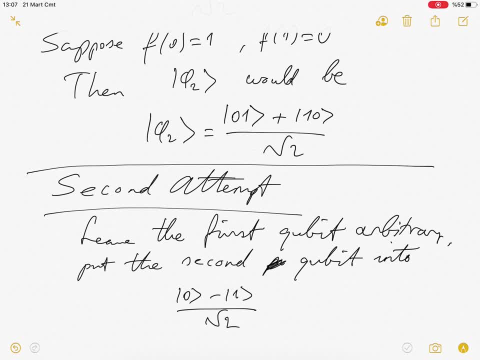 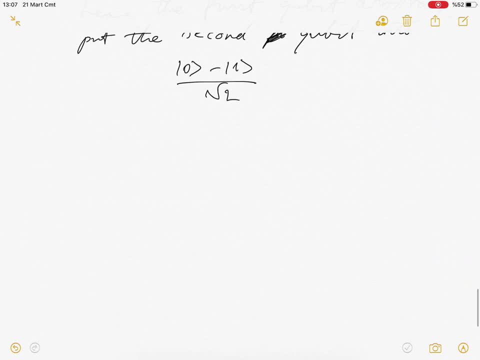 that is ket 0 minus ket 1 divided by square root 2,. okay, So let's draw the diagram. We have uf. The first qubit will be arbitrary, so let's call it x The second qubit. we'll start with ket 1,. 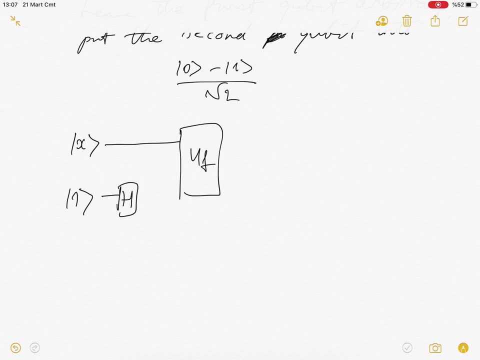 and then we apply a Hadamard transform, because h1 will be equal to the minus phase superposition state. And then we have output wires and let's again measure the first qubit. Okay, So let's call the state phi 0,. 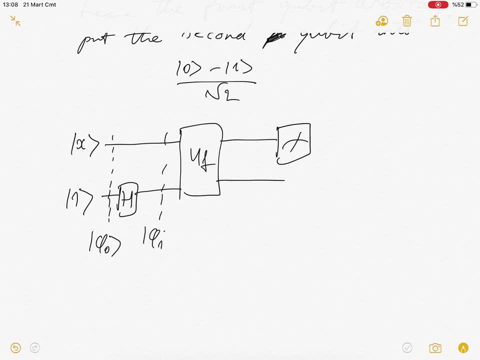 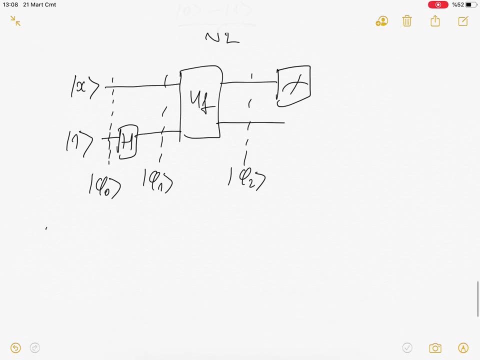 and let's call the next one phi 1.. Let's call this phi 2.. Okay, So it's immediately clear that phi 0 is basically x1.. The first qubit is in an arbitrary state that we don't know. 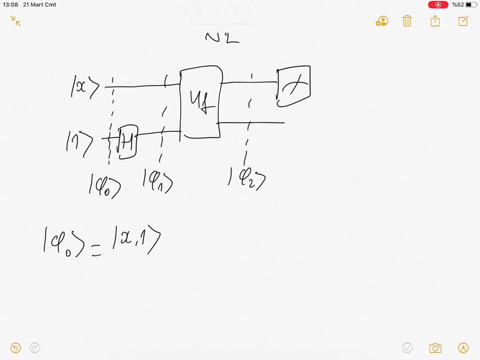 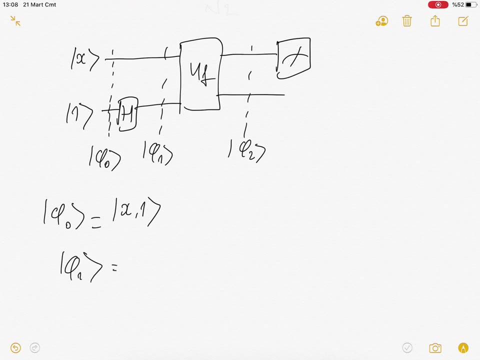 and the second qubit will be arbitrary. And the second qubit will be in state 1.. So we start with phi 0.. Phi 1 will be The first qubit changed. It remains the same tensor. The second qubit will be in the minus superposition state. 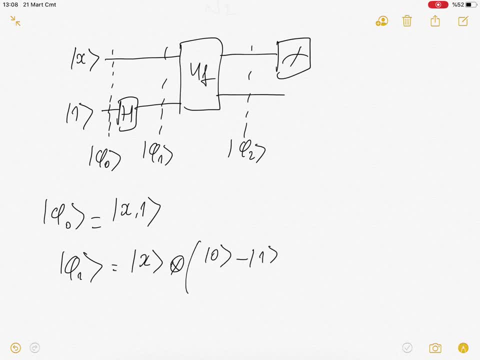 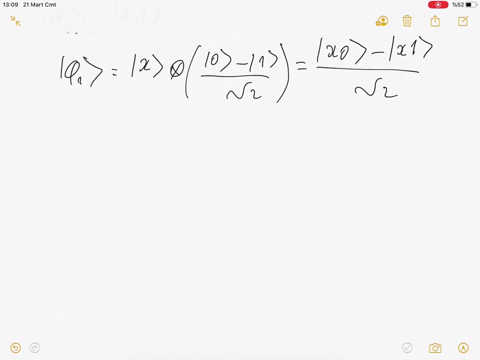 ket 0 minus ket 1 divided by square root 2.. If we distribute this, we get x0 minus x1 divided by square root 2.. Okay, So now we apply UF to the state, Again by linearity. 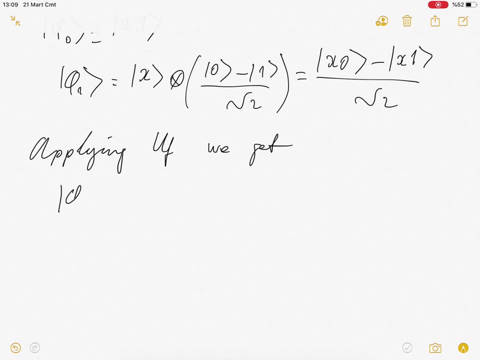 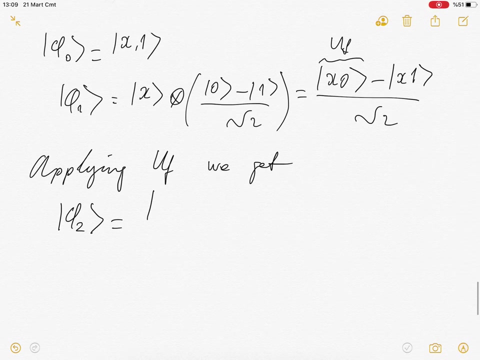 So let's take a look at the first component here. If we apply UF here, Okay, That means the first input to UF is x, the second input to UF is 0.. Well, this will be. The output will be x, 0, xor f. 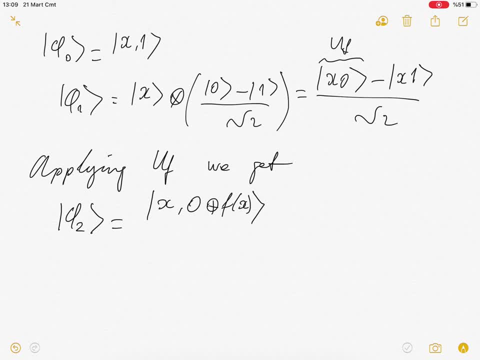 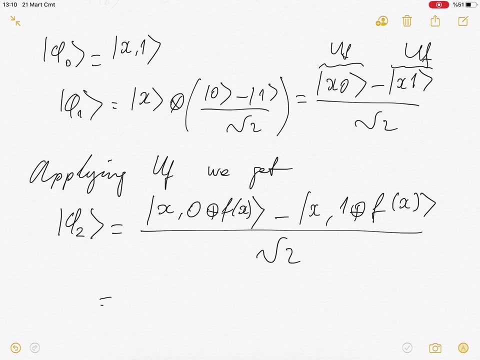 f, All right, And then we do the same thing to here, And this will be equal to x1, xor f, And then we have the common factor 1 over square root 2.. Okay, So this will be actually equal to. 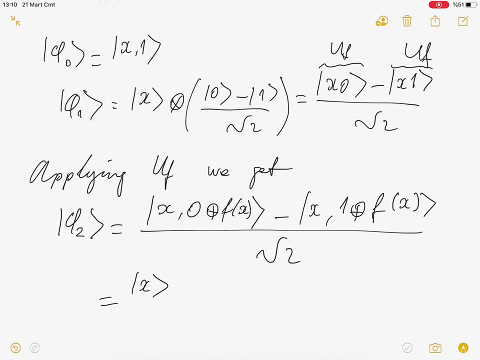 Let's take out x. x will be our first qubit And the second qubit will be in a superposition, f minus the complement of f, Right. So this will be Complement divided by square root 2.. Okay, 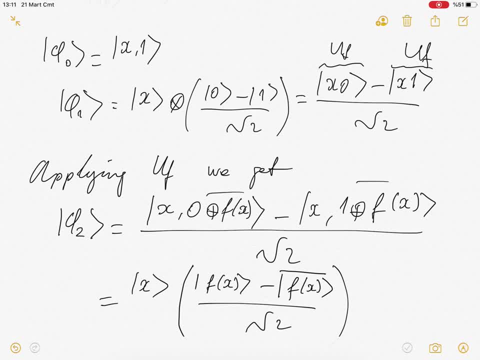 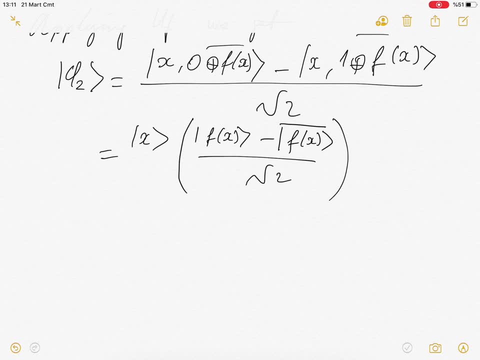 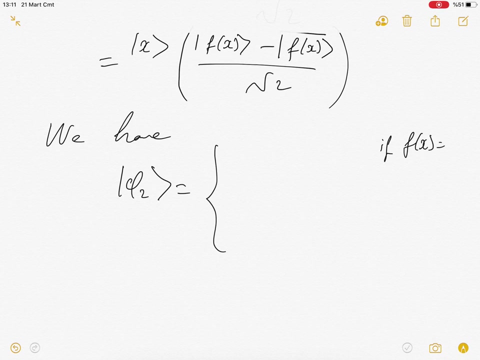 Because these will be complement of each other. All right, These two components, Okay. So depending on the value of f, phi 2 will be in one of the two states. so let's draw an array, okay. so if if X, if f of X is equal to 0, then Phi 2 will. 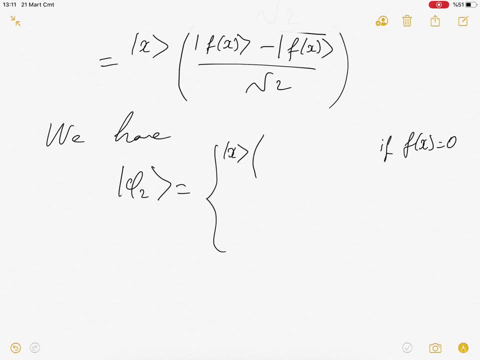 be equal to cat X tensor 0 minus 1 square root of 2. but if f of X is equal to 1, then we have the same superposition state, the same 2 qubit superposition state, except that we have 1 minus 0. 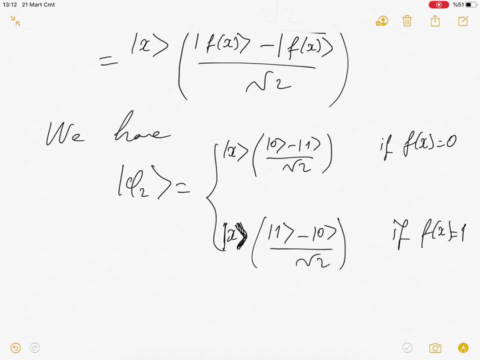 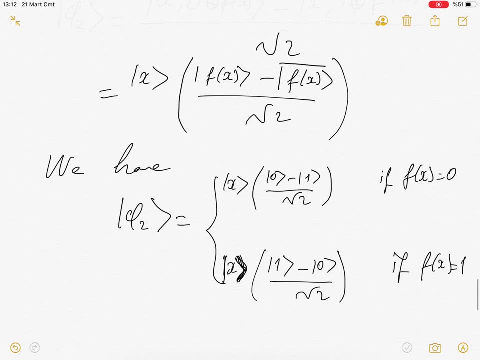 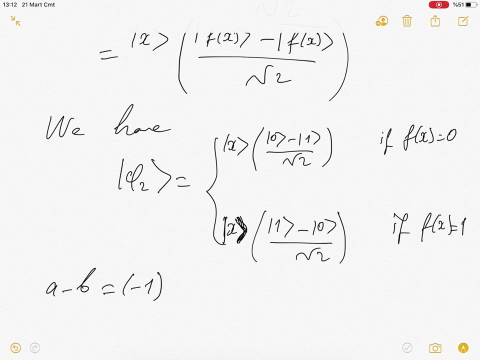 square root 2. okay, now, by simple algebra we know that a minus 1 can be written as minus 1 times B minus a. okay, let's. I mean, if we look at the second qubit of Phi 2, they're actually a minus 1. 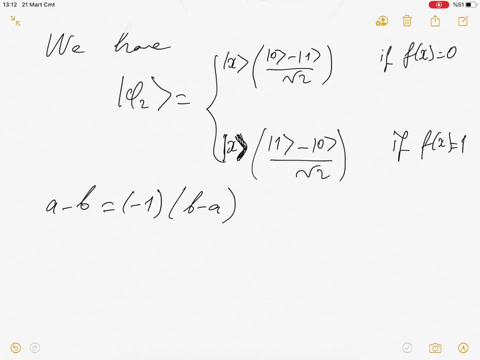 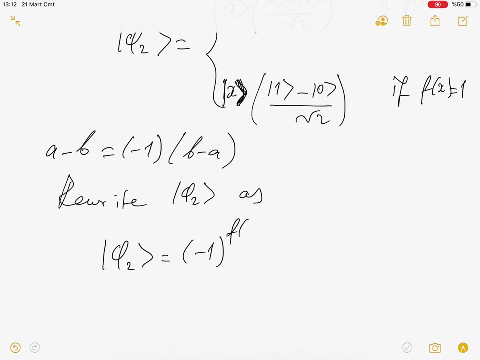 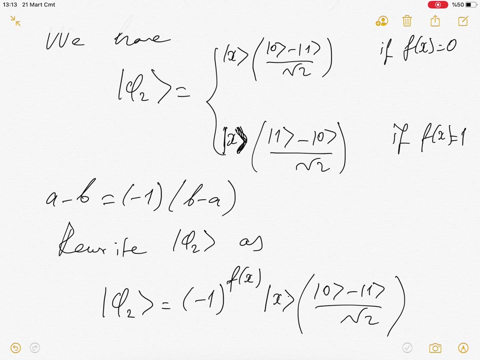 multiplication of each other. okay, so we may rewrite Phi 2 as minus 1 over f of X as a factor, and then we have X tensor 0 minus 1 over square root of X. okay, so if f of X is 0, okay, then this will be. this will be plus. 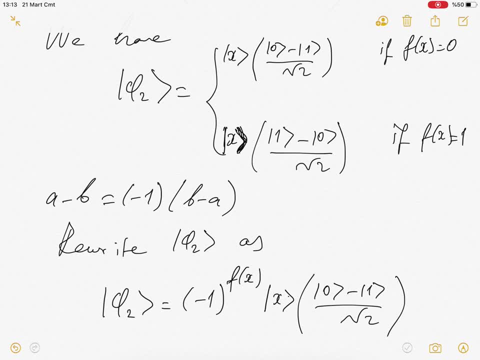 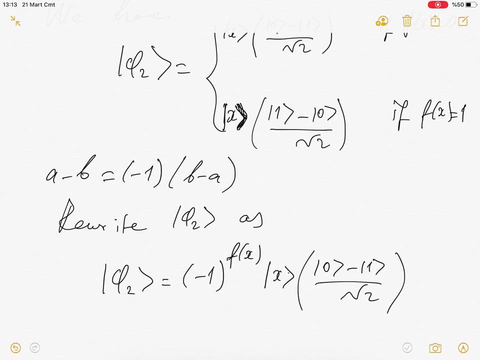 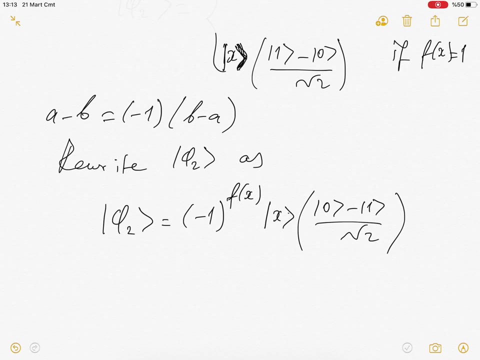 1, and then we have X, this superposition. but if f of X is what? if f of X is 1, then we have a minus 1 factor, minus 1 amplitudes, and then the order will be changed in the second qubit. all right, so what happens if we measure either the 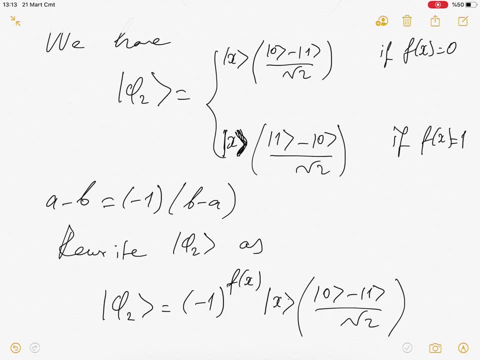 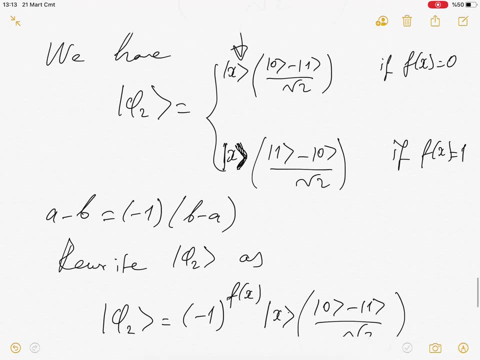 first qubit or the second qubit? okay now, if we measure the first qubit, it's in an arbitrary state, right, it can be. it could either be 0 or 1, so we have no information about the first qubit. and if we measure the second qubit, well again. 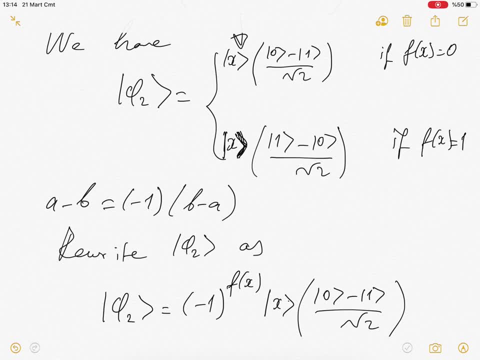 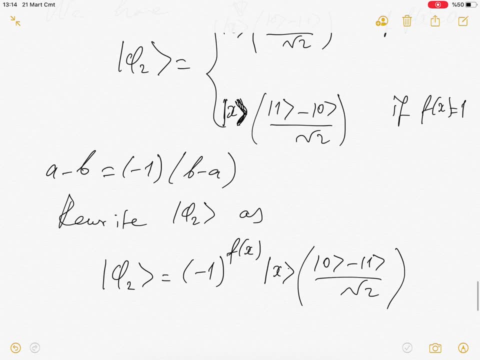 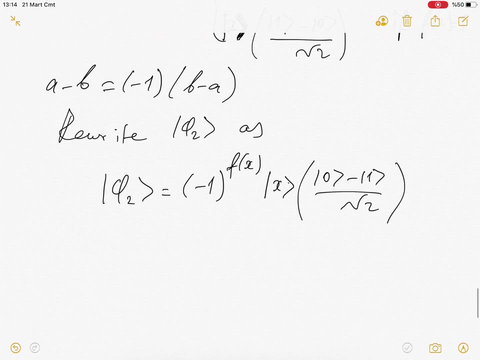 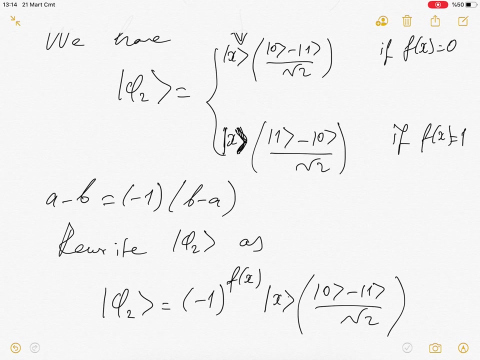 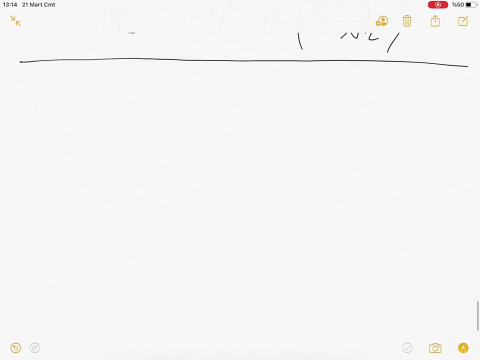 it doesn't give us any information. right, it could be in either one of the superposition state with the same probability, okay, okay. so the second attempt also fails because it gives us no information about the characteristic of the function f. all right, so finally, I'm going to give the solution. so now, 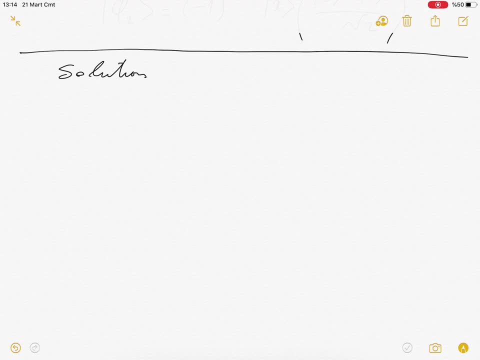 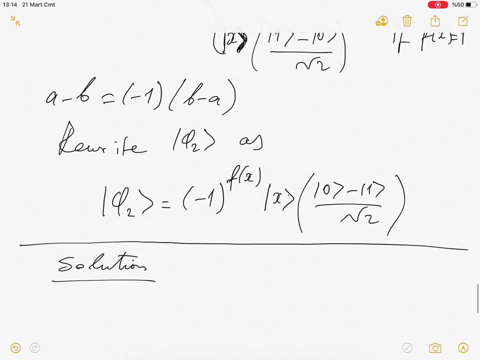 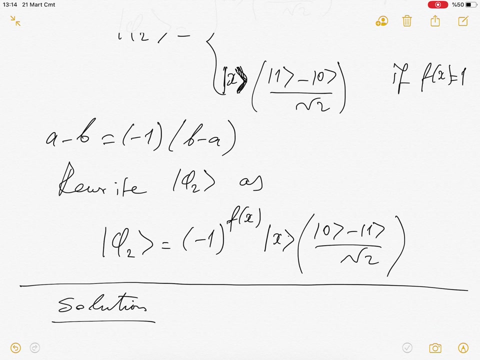 the solution. you all right. so first note that when the second input to the Oracle UF is: is the minus state superposition, okay then, in fact the output of UF shows a kind of kickback characteristic here. okay, so we have a. so this vector is actually the eigenvector of UF. the eigenvector of UF. 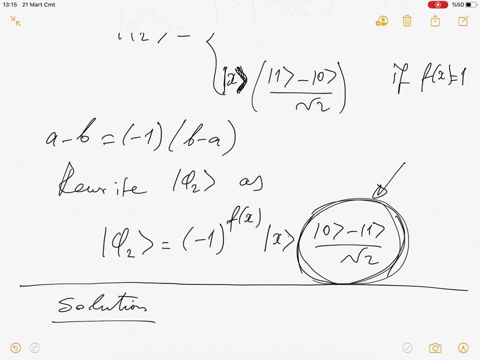 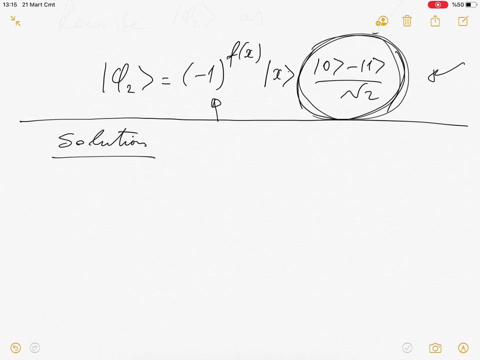 because if the input is an X and Y and Y is equal to this negative phase superposition state, then the output will be the same, except that we it picks up the phase of minus one. okay, now we will use this property in the solution. Okay, so let's put first and second qubits into superposition. 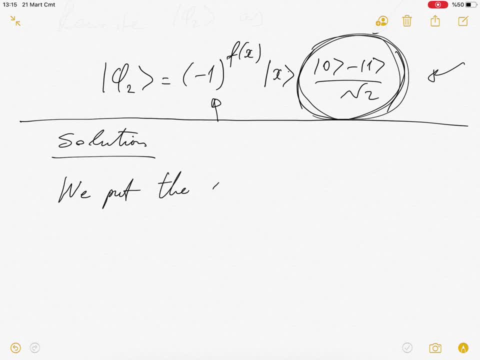 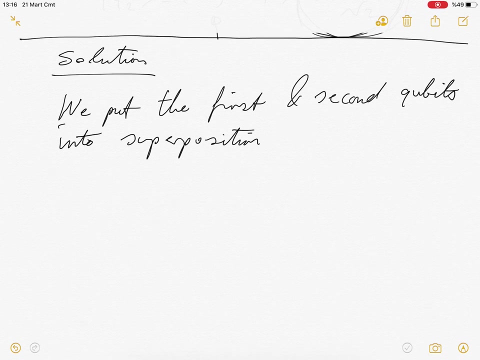 We put the first and second qubits into superposition. But not only that, but we will also put the output into superposition. that is, we will also have a Hadamard transform in the first qubit of the output wire of UF. 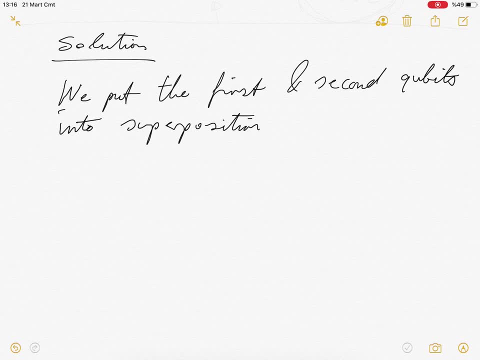 And the quantum circuit will be defined as follows: We will start with zero. we will put a Hadamard transform here, okay, and this will be our oracle UF. And then the second qubit. we will start with one. We put a Hadamard transform. this will be the second qubit. 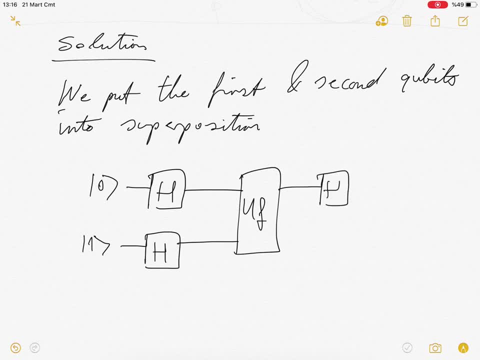 And in the output we put another Hadamard transform in the first qubit of the output And then we make a measurement. So we only need to measure the first qubit. that will be sufficient. All right, so let's denote the states. 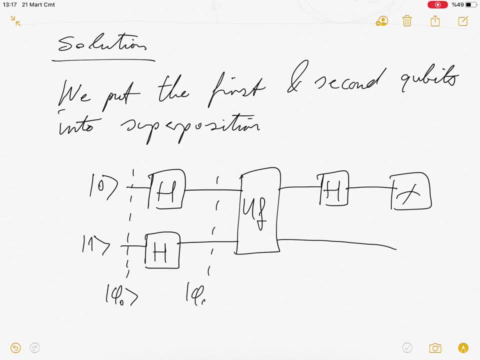 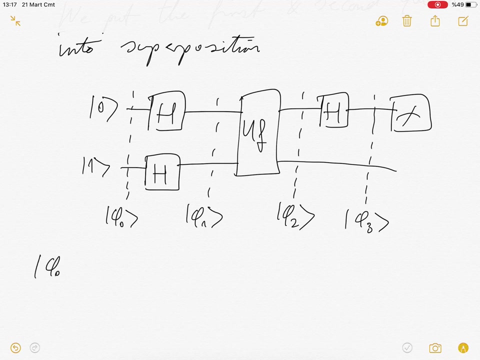 Let's call this phi zero. let's call this phi one. let's call this stage phi two. let's call this phi three. All right, so let's now examine these states. Let's write them explicitly. So obviously, phi zero is equal to. 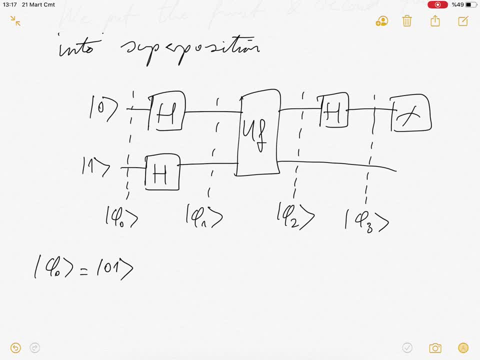 state zero, one right, And we apply the Hadamard transform on both qubits, but that means that both qubits will go into superposition. So zero will be transformed into zero plus one divided by square root two. okay, So this is simply Hadamard zero. 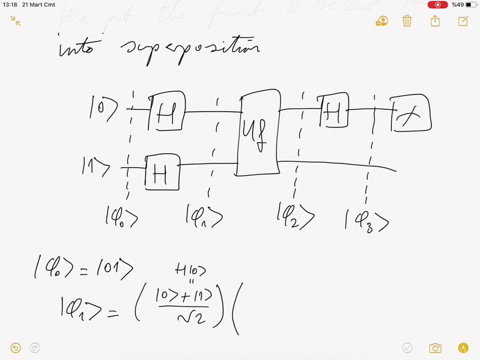 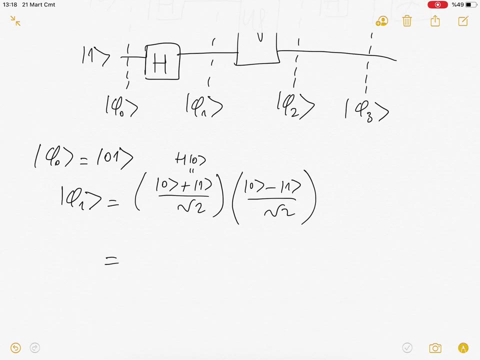 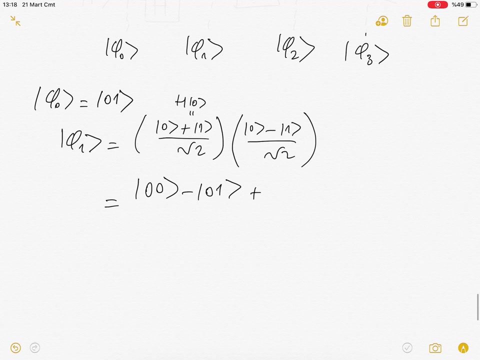 And then we have in the second qubit, we have the negative phase, superposition, Hadamard one. All right. So in fact this will be equal to, if we distribute it, zero, zero minus zero, one plus one, zero minus one one. 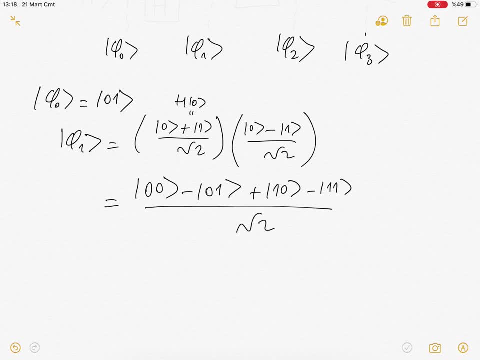 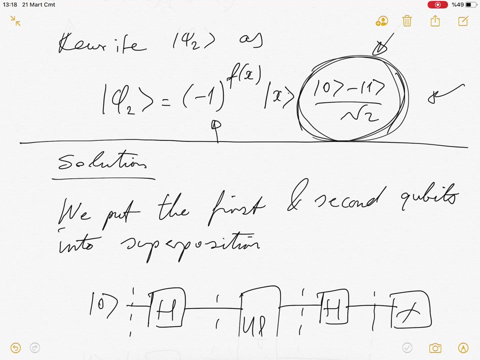 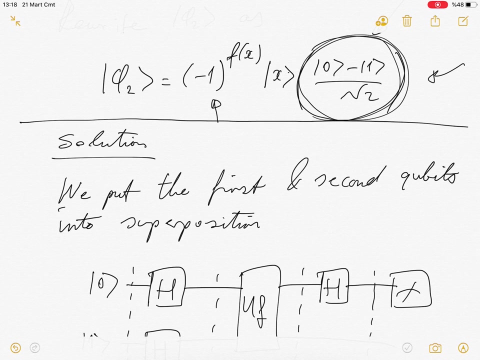 So this is equal to zero. zero one plus one. zero one plus one. zero one plus one. zero one two. All right, Now we saw earlier- I just said a minute ago- that when the input of Uf, when the second input, is the negative phase superposition state, then the output will be simply one. 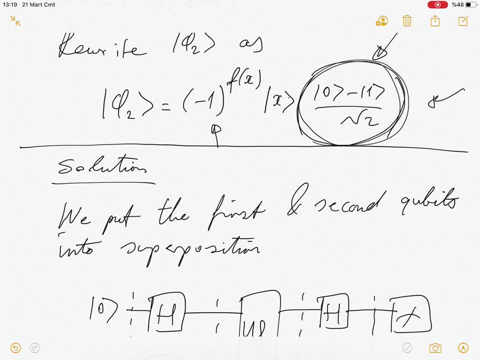 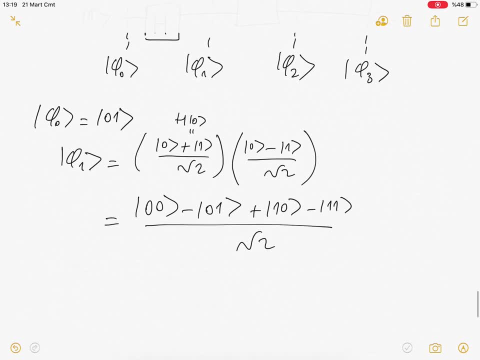 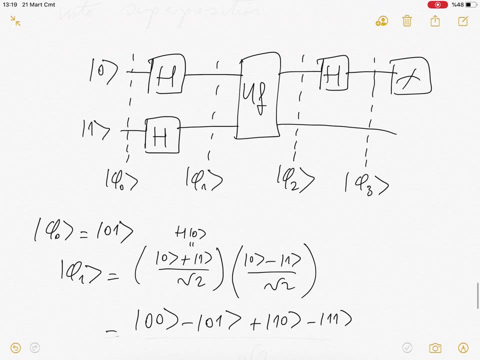 So this is actually minus one over f of x, right? We have this phase, So we have the same situation here. Okay, The second qubit of phi one is the negative phase superposition, right? So this is actually the second input of Uf. 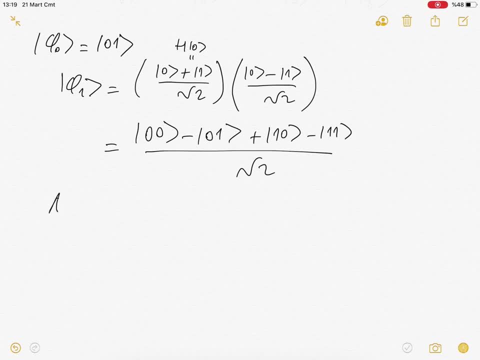 So then. So let's write this as a note. Okay, All right. So, in fact, zero minus ket, one over square root. two is the eigenvector of Uf with eigenvalue minus one over f of x. Okay, But now. 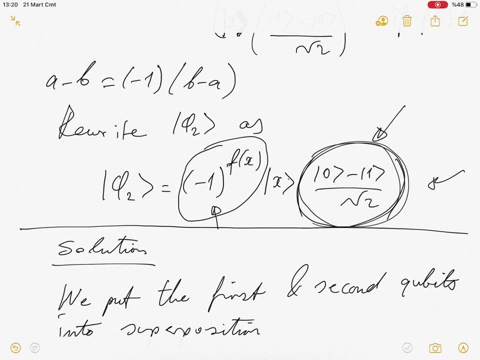 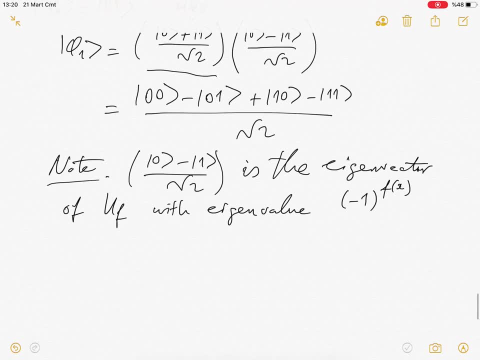 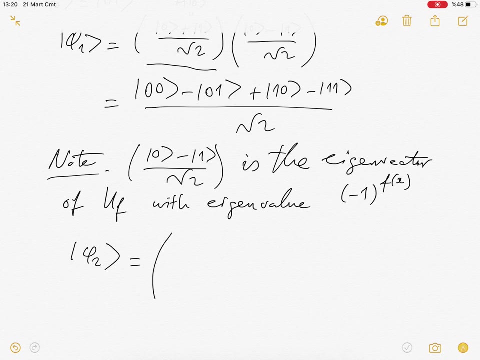 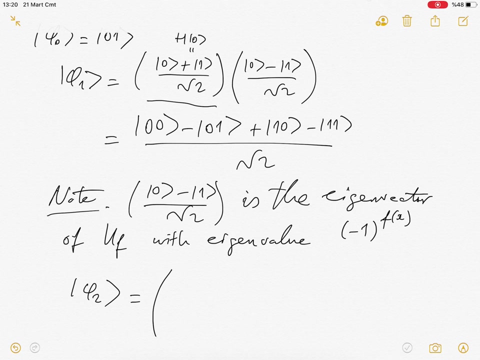 Now we have x: Okay, So x is in the superposition right. Let's rewrite phi two, So phi two will be equal to okay, so x is in the superposition state. and then we have minus one over f of zero. 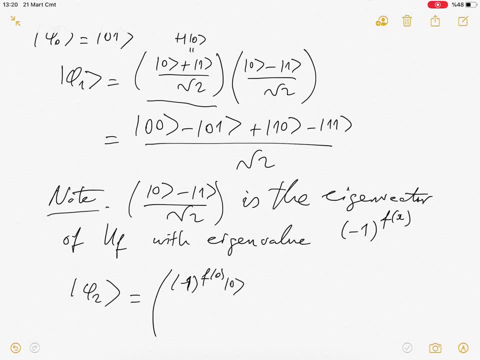 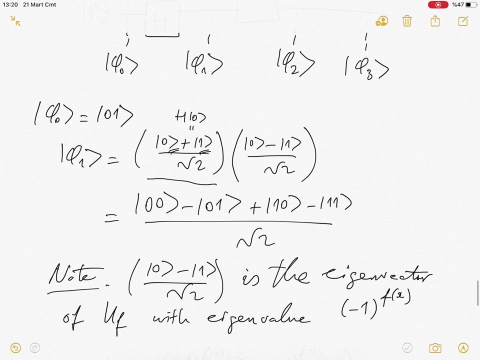 Okay, So we write one for ket zero and one for ket one. Okay, Plus minus one over f of one over ket one divided by square root two. So this will be the first qubit of phi two. The second qubit will remain the same. 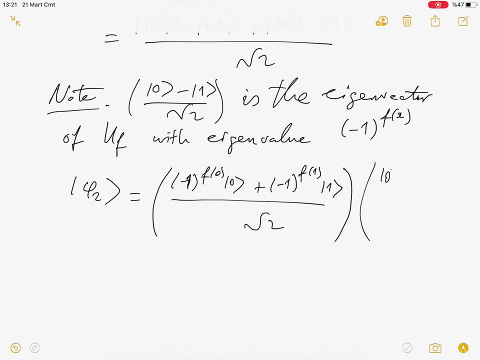 It's still the superposition state. Okay, It's still the superposition, the minus state. superposition Zero minus one divided by square root two. All right, So let's now take a look at the numerator of the first qubit. 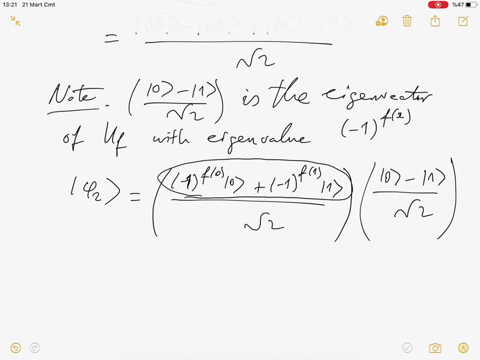 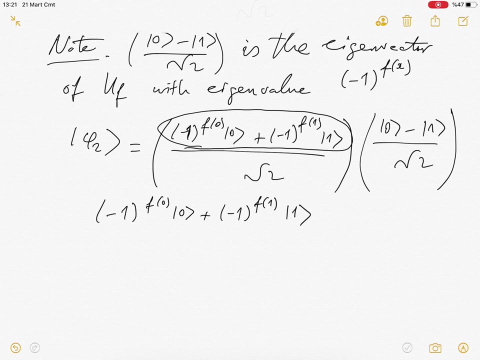 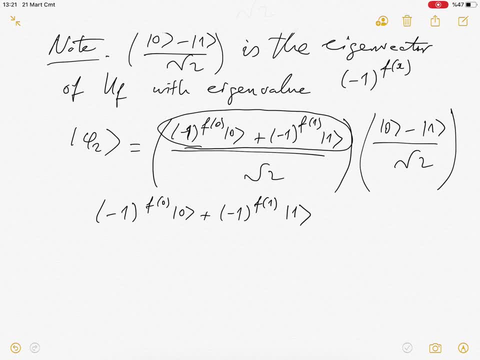 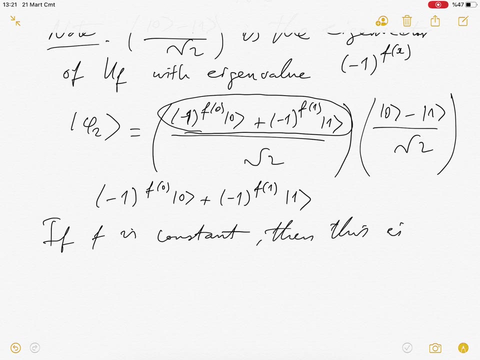 two. Now, if f is constant- If f is constant, then the above expression then is negative. then this either becomes plus 1 times plus 1 times 0 plus cat 1, or it becomes minus 1 cat 0 plus cat 1. right, so, depending on how F is defined. but if F is constant, 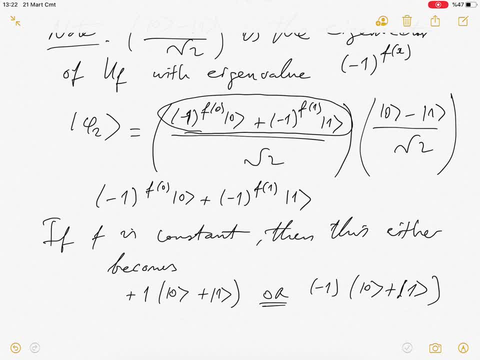 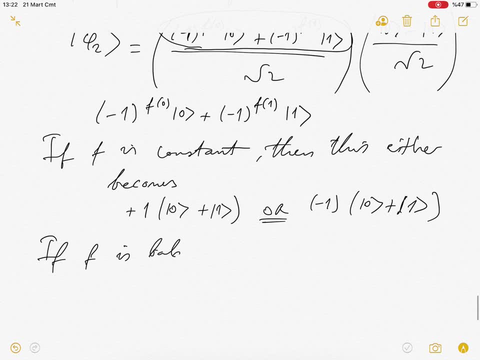 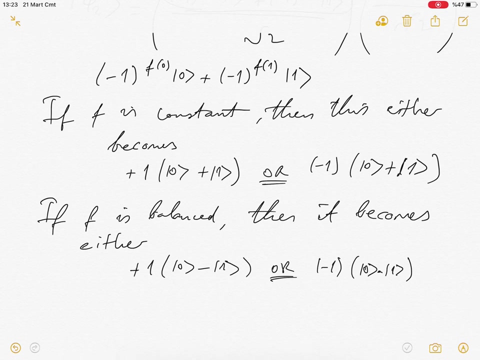 it's going to be this, this expression will be equal to one of them. but if F is balanced, well then it becomes either either plus 1, 0 minus 1, or it becomes minus 1 times cat 0 minus cat 1. okay, so if F is balanced, we actually have the same state, except the face, and if F is, 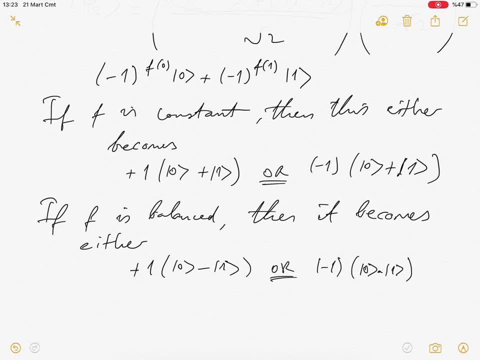 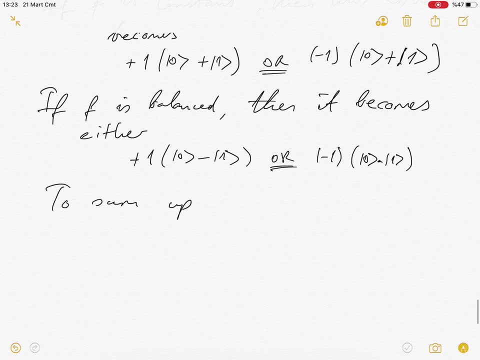 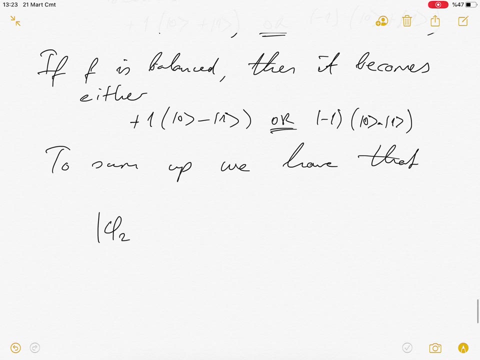 constant. we have another state with possibly different phases, so let's sum this up. to sum up, we have that. so Phi 2 will be either you plus minus 1 times cat 0 plus cat 1 divided by square root 2- this is our first qubit, and 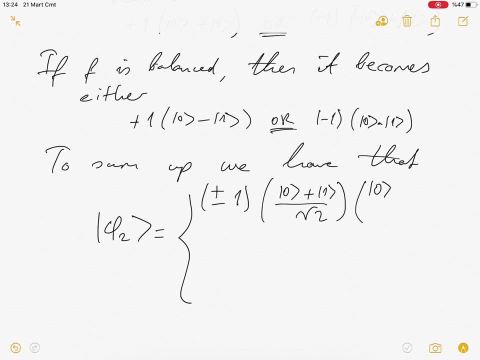 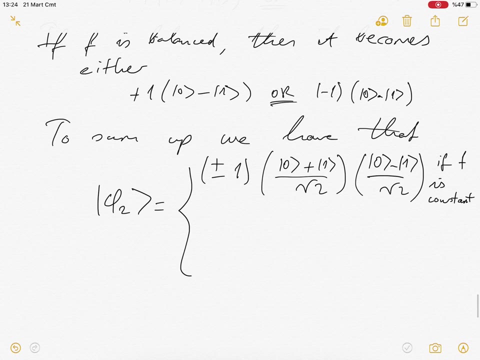 second qubit will be 0 minus cat 1 divided by square root 2. if F is constant, okay. if F is balanced, then we have plus minus 1 times 0 minus 1 divided by square root 2. second qubit will be the same. 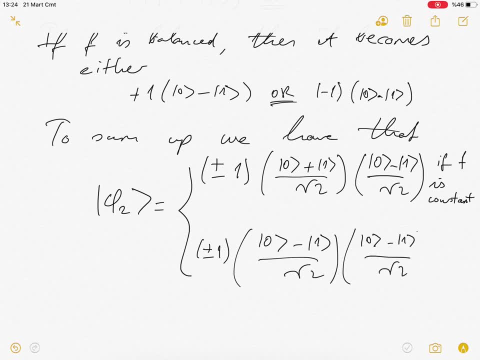 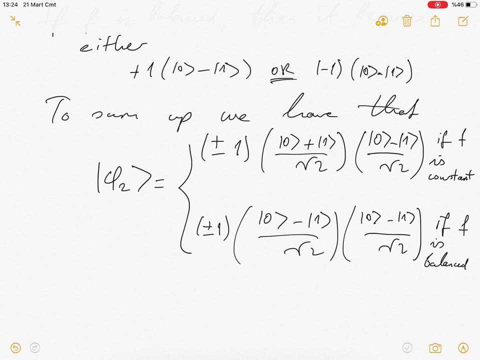 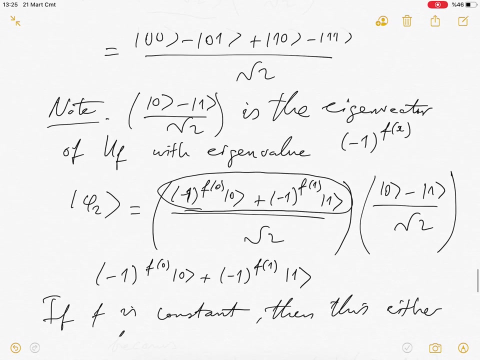 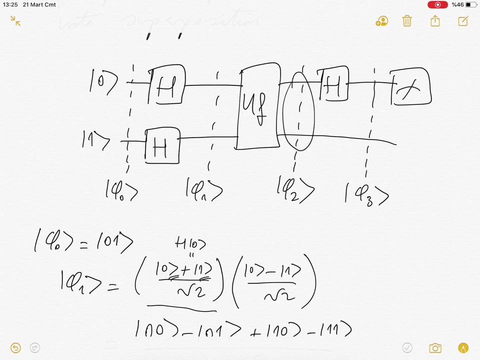 and this is when, if F is balanced, alright, so Q2- sorry, Phi 2- will be either one of the it will be in in one of the states, depending on whether F is constant or balanced. okay, alright. so here comes a trick. the trick is to apply a Hadamard transform on the output of the first qubit of uf. 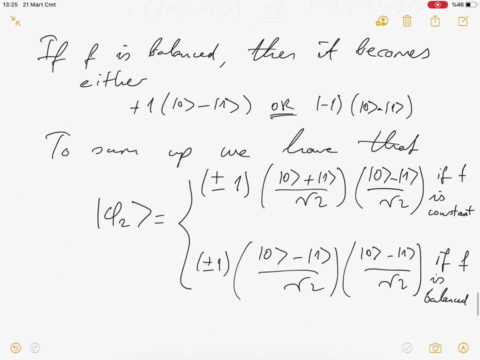 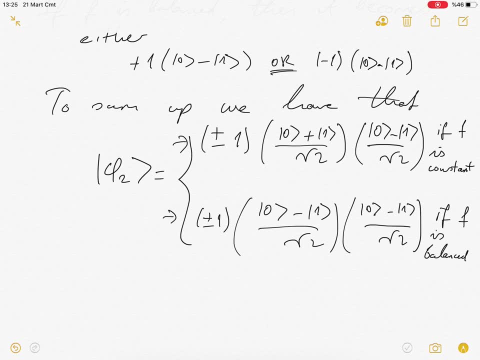 so we are here now, okay, Phi 2 and depending- okay, depending on whether F is constant or balanced, it's in either one of the two states And we're going to apply a Hadamard transform on the first qubit. okay, on the first qubit. 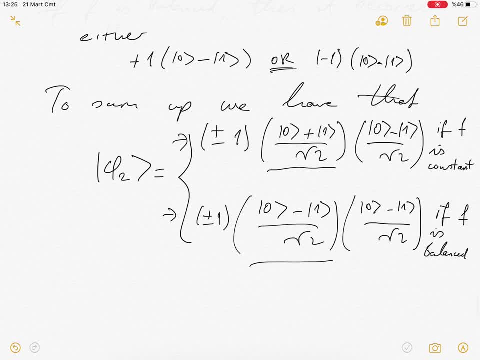 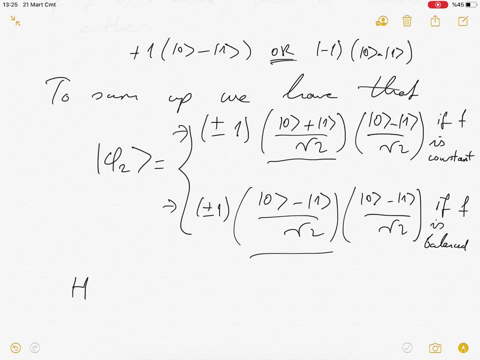 of phi 2.. So what's going to happen is that Hadamard transform is its own inverse, okay, That is, if we apply Hadamard 1, if we apply a Hadamard transform on Hadamard 1, we get. 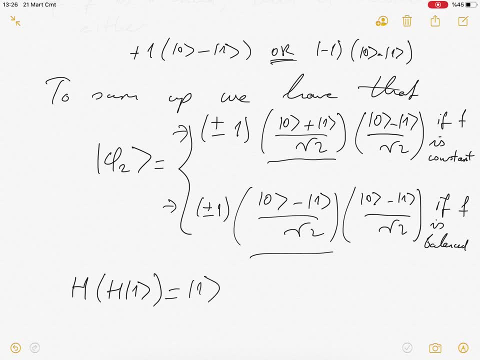 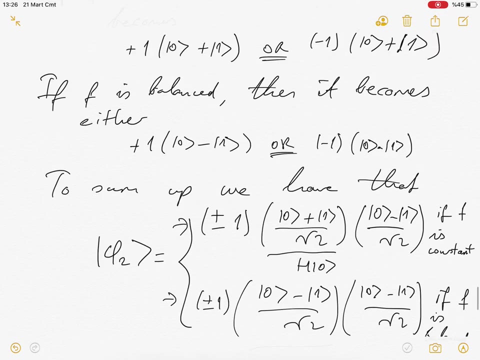 1.. And similarly, if we apply the Hadamard transform on H0, we get 0.. Now, so this is what this is actually: Hadamard 0. But if we apply Hadamard 0,, if we apply the Hadamard gate, the Hadamard transform here, 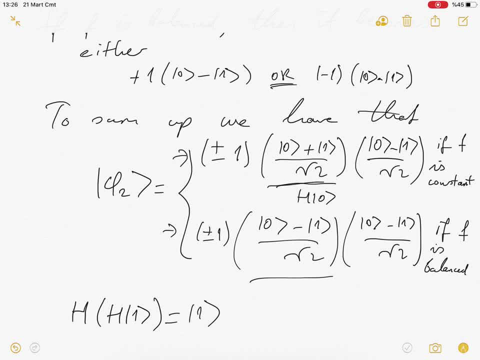 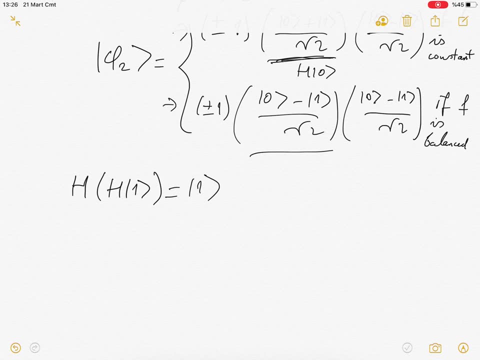 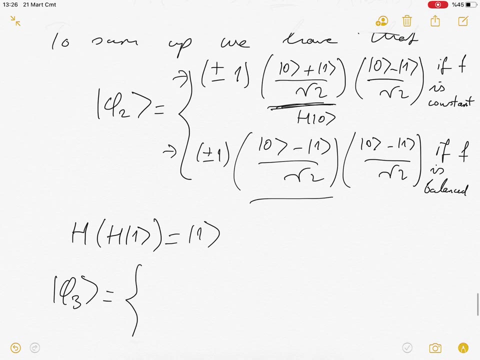 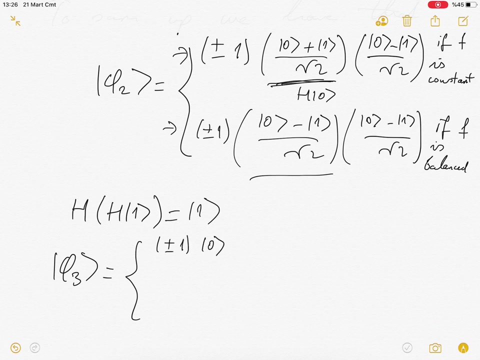 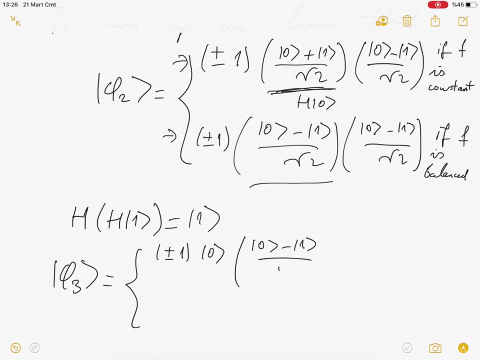 okay, On this superposition state. well, we get 0, right, So let's write phi 3.. So phi 3 will be: it's either going to be plus minus 1 times cat 0. Or it's going to be minus 1 divided by 0. 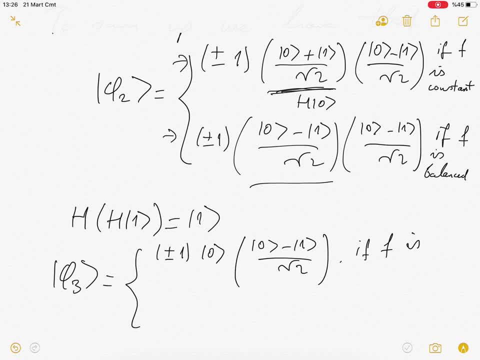 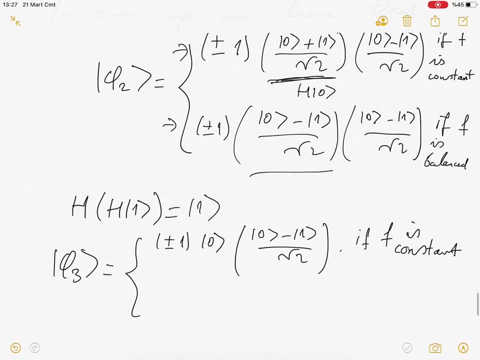 So this is: if F is constant, okay. And then if F is balanced, if we are in this superposition state and if we apply the Hadamard transform on the first qubit of phi 2, so this is already Hadamard 1, and if we apply